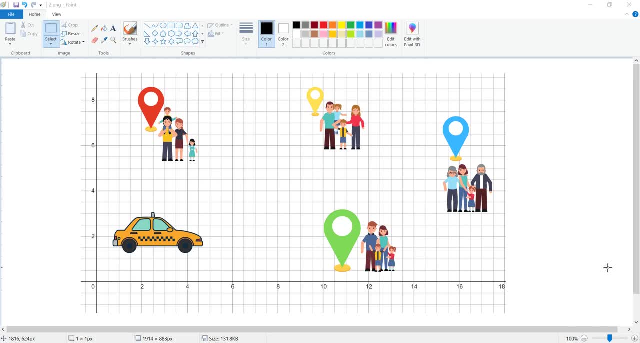 Hello people, welcome back to my channel. So hope you're enjoying the Python skill series so far. So we have covered so many videos in Python skill series. We have implemented some of the machine learning models. We have seen some of the deep learning models. Now in today's video we'll be basically creating a reinforcement learning environment and we'll be basically implementing the Q learning setup that we have seen in the conceptual video of reinforcement learning. 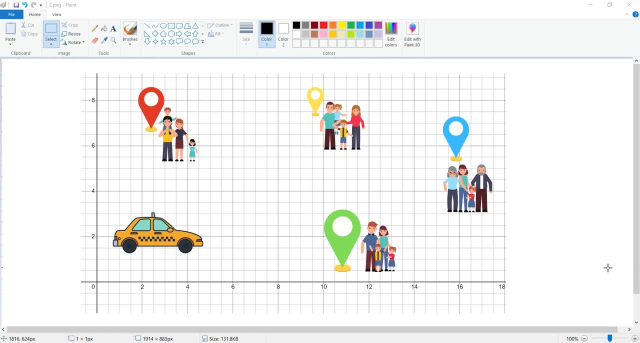 So in the last video we saw what was the Q learning approach, what are the mathematics behind it and what are the different concepts and terms which are there in Q learning. Now, if you have any doubts regarding that implementation video or the conceptual video of Q learning, I suggest you to watch that video. And if you still don't understand that video, then we'll do a small. 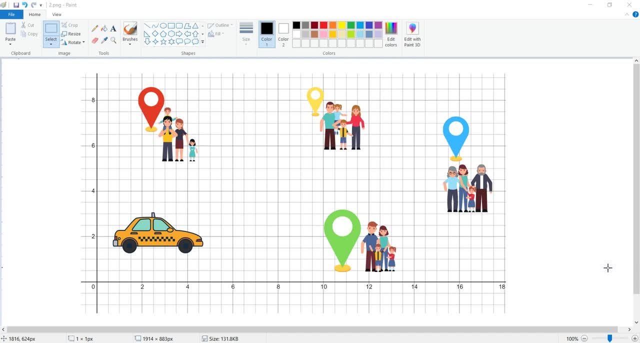 implementation of that Q learning in this video, So you can have a better idea of what the Q learning algorithm is and how the different parameters or the entities fits into place. Okay, so for this particular example for Q learning, what we have is a. we have an environment, So we always love to spend time with our families. So 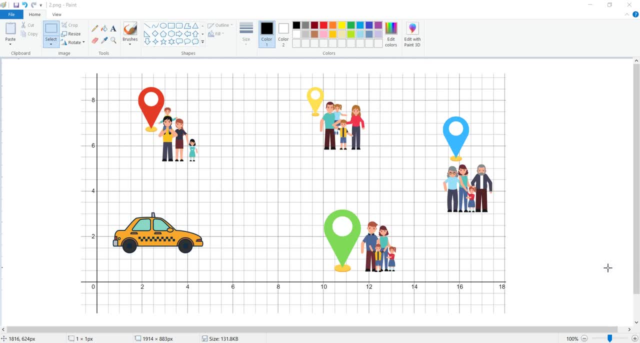 say, we are at a park and at this particular park we have some certain locations. So the locations are R, then yellow, then blue and then green. So you have four different locations and there are certain families who have come to visit that particular place on a particular day. Now our major goal is to design a taxi that is, an autonomous. 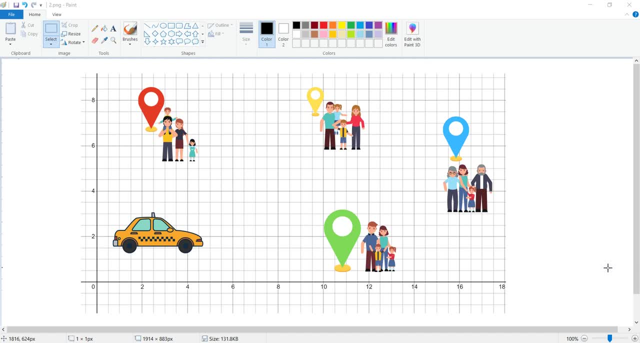 self driving taxi. Now, in the real world, there are this kind of things there, But it's not full fledged out so that it can be made available into production. So there are some issues with this kind of models or with this kind of agents. So we'll be just having a touch base over these techniques, how it is actually implemented. 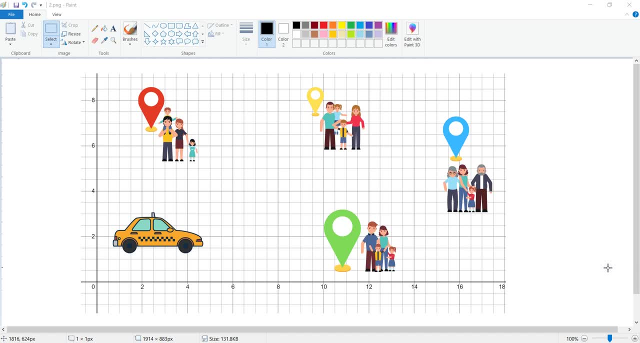 Just a small overview of this in this particular video. So our aim is to create a taxi, which is this one. So now, this taxi here is not controlled by a human being, but instead it is being trained by a reinforcement learning algorithm. So the algorithm or the technique that we'll be using- 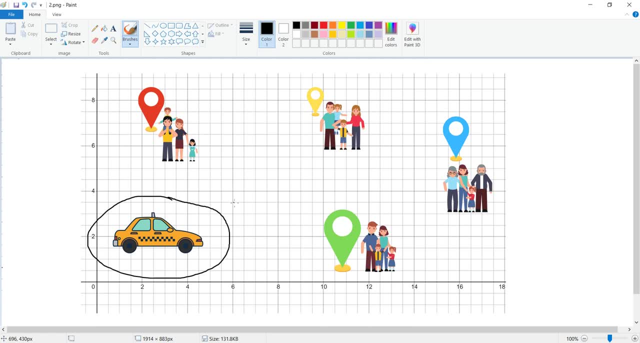 is Q-learning. quality learning means it has to go to that particular location where the customer is or where the user is, Then it has to pick up these many people, or how many people are there, And then it has to basically drop at some particular location where the user has requested to. It can be this blue location or yellow location or green location, It can be vice versa, So it 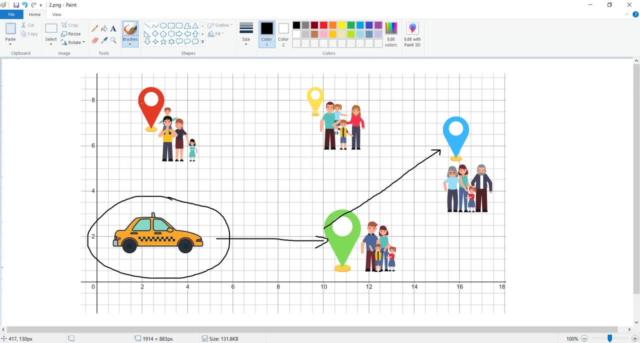 can be. one is to one, So there is only one smart taxi available at this particular picnic spot so that it becomes easier for their pickup and dropping. So we want to design this kind of thing using reinforcement learning. So what we have is we have a library, So that is called as gym. All right. so gym is an open AI library where you can create different reinforcement learning agents, as you can see here, So where you have different kinds of libraries and open environments that are available, from where you can build this. Now, just mind you, the codes that we are using in this are taken from this, So everything we have got here is agsulliappil solventylog. thisньviz 고무리. 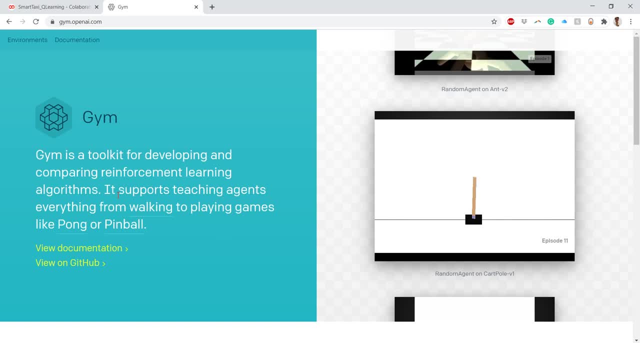 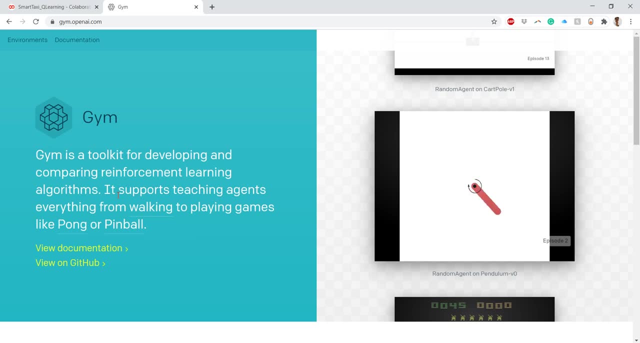 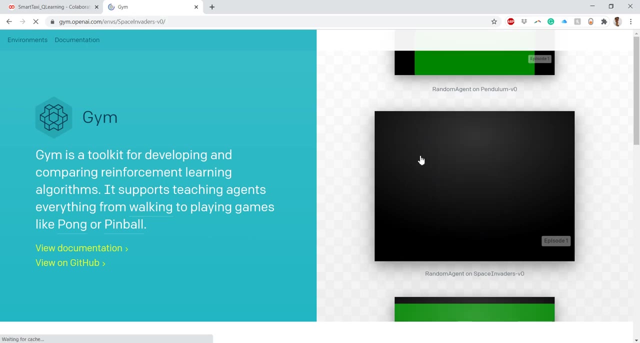 what I show. it's not created by me, just a demonstration of the pre-existing environment. so from that we'll be just seeing how the things are basically done and how you train these agents in that particular environment. so you can see, here there are different kinds of 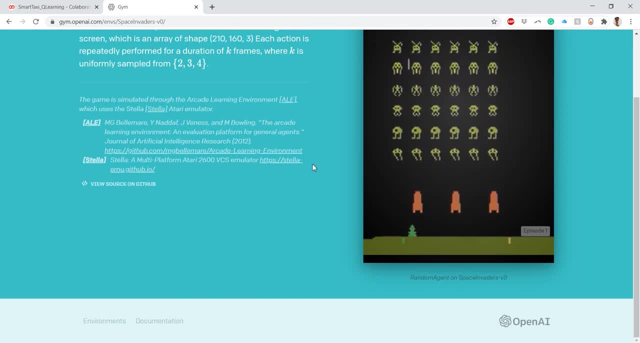 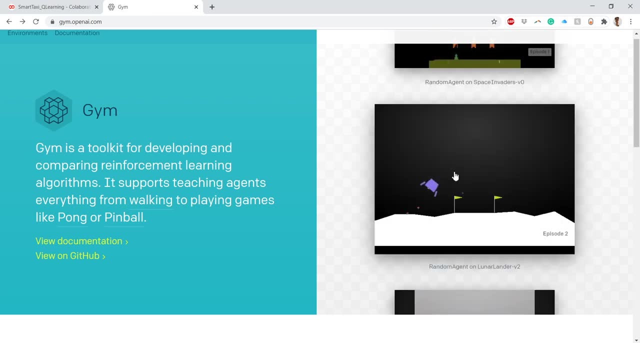 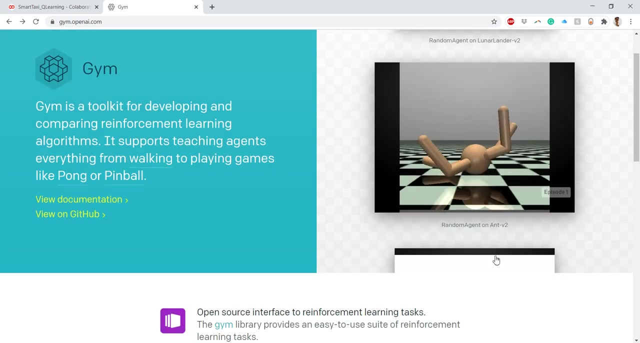 scenarios or environments that are there so you can find this source code from this particular website. then many different things that are there: lunar agent, then you have something like this, and then you have a cart pole, then you have a pendulum- so many different things are there. I. 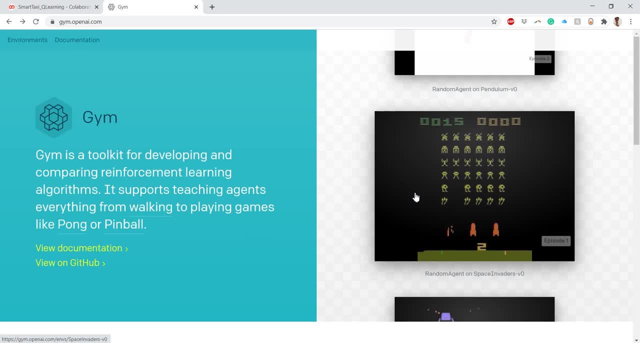 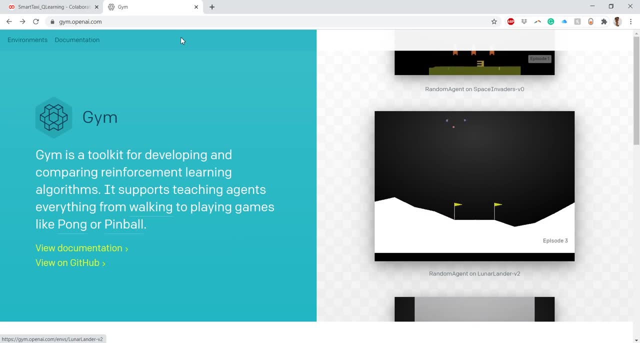 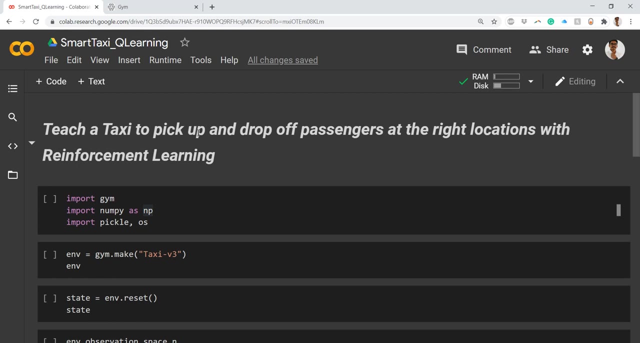 suggest you to check this link out. if you have any doubts regarding this, or if you want to implement anything, you know you can go here and just implement this. okay, so back to our discussion. we want to you design a smart taxi using Q-learning. so how do we do this? so we want to teach a taxi to pick up. 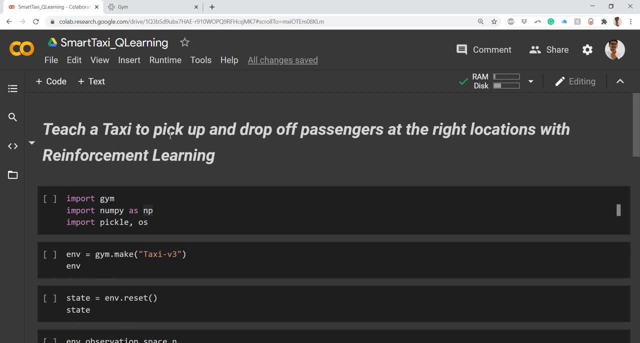 and drop off passengers at the right locations using reinforcement learning. so we'll be using the Q-learning approach here. so first we'll just initialize the variables and just we'll do a initial run how we can do this. so for that we have to import certain libraries which are 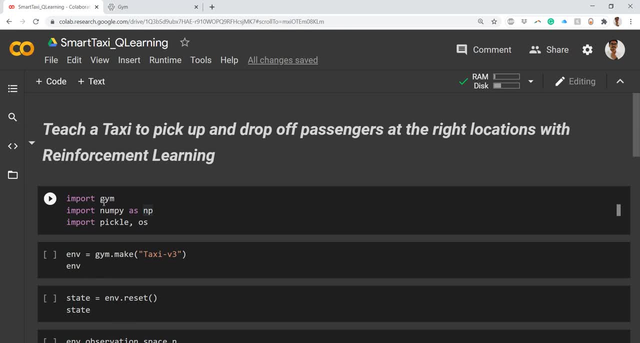 pertained to only reinforcement learning. that is, we import the gym library. so in gym library there are pretty much rich kind of other methods that are available so that you can build an environment and you can train an agent in that particular scenario. and then we basically using numpy library 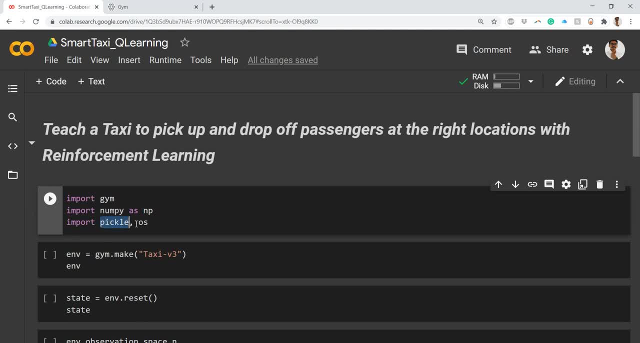 and then we have the pickle. so pickle, we have seen that is for object serialization. and then we input the os library for doing some input and output. okay, so first what we do is we just import this libraries and we just initialize the environment here. so what I do is from the gym. 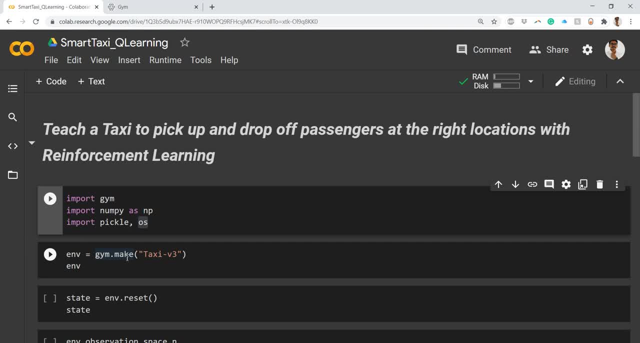 library I am importing or calling the make function. so in make what I'm passing is I'm passing out a environment. now this taxi v3, that is, taxi version 3, is already pre-existing. so I am just using the already pre-existing library which is present in the gym and I am making use of this and then I am trying. 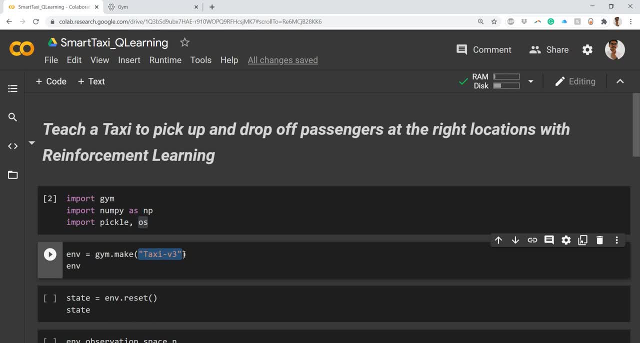 to train my reinforcement learning agent so that it can pick up passengers and then drop them off at a particular location, so that I am storing in a variable env. so you can see. I have just printed the env variable. it's a time limit- env- taxi. env- taxi version 3. so there are different versions. 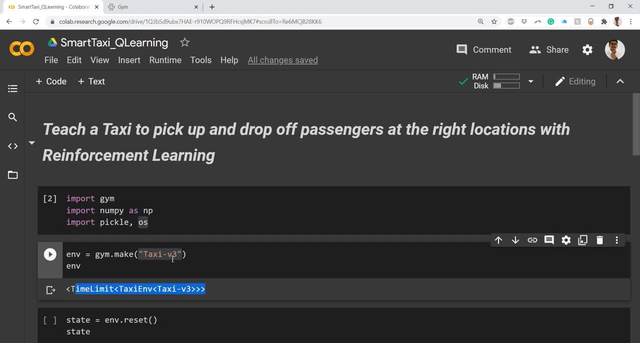 of this environment, like version 2, version 1, version 3, so they keeps on updating different parameters and all these things. now, just mind you, all the other graphics and all the constraints and all the parameters are all the same. so I am just printing the env variable and then I am. 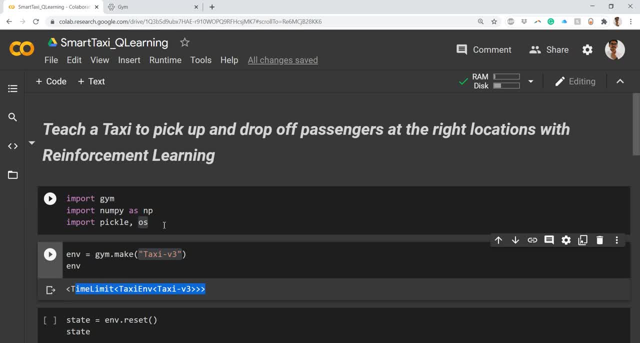 particle, which are there in the path of the agent, are defined in this particular library. so if you want to see the source code, you can see the source code. we are just going over this: how this particular scenario looks like. then what I have is I just define a state. 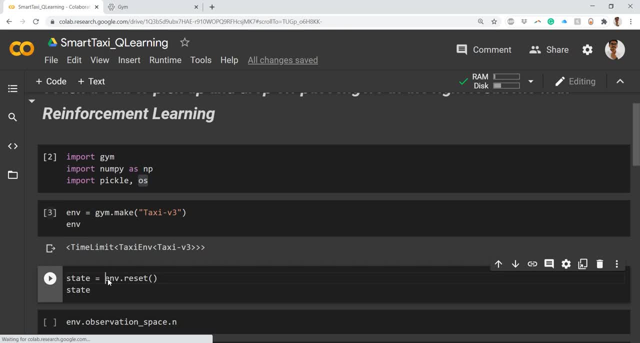 so what I am calling is on the environment, which is already there. I am resetting the environment. so why resetting is done? because it resets the state of the environment, as you can see here, and returns the initial observation. so when you initially load this particular environment, there may be something. then you just reset it to the original state, so that what previously it was, 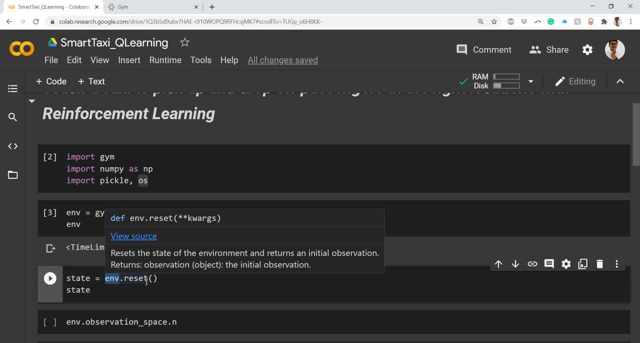 there. it will use those libraries and not the one which is updated at the very first run. so we are basically clearing of the environments and libraries so that we can have a better training of the agent. so we are doing everything from the scratch from this particular environment. 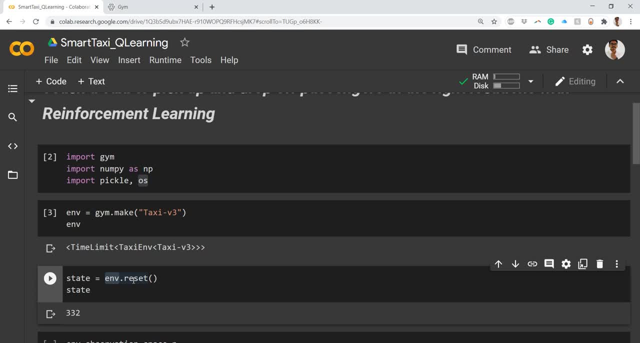 okay and I just run this and the state when I printed it came out to be 332, 32. now we know, like in reinforcement learning, our basic building blocks are simply three blocks, so we can just save the state of the environment and then actually create the new state in it, and then we can actually test our environment and we can also use their. 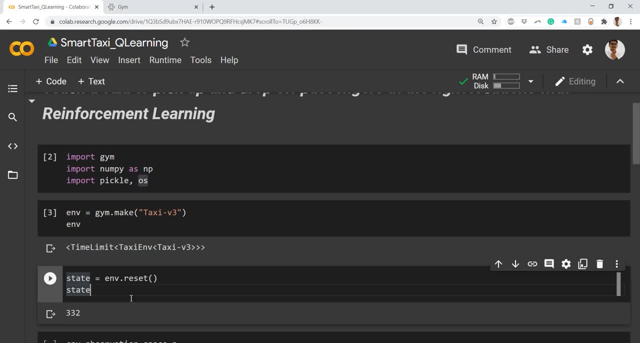 states and actions. then we have rewards, then policy and all these things. so we'll have those things here. so states are nothing, but how many different states are there in that particular environment? so that is 332. so now you might have observed this value keeps on changing. 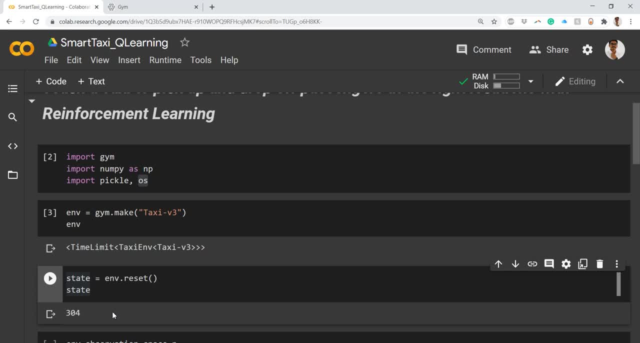 yes, this obviously keeps on changing because dynamically it is being updated every now and then, so that's why you get different values when you run each time. so you have to, just so it keeps on changing from lower number to higher number, as in when you just run this again. so it 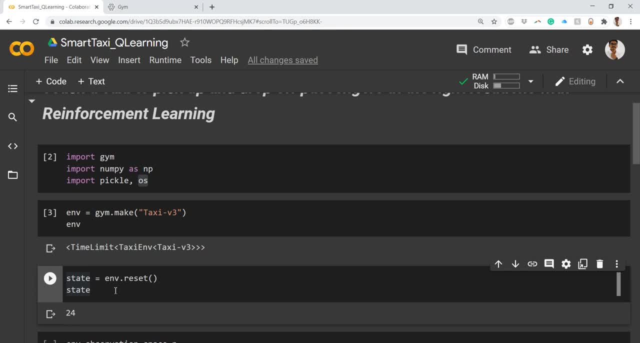 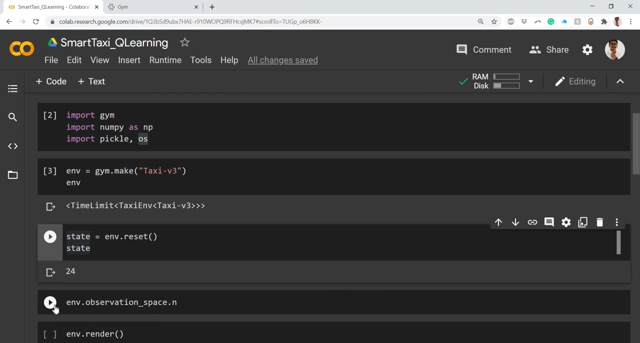 also depends upon the other parameters also. so that is a kind of little uncertainty present in this reinforcement learning. that's why you have to train this agents and models again and again. okay, so then we do the observation space. so from the environment we see the number of observations. 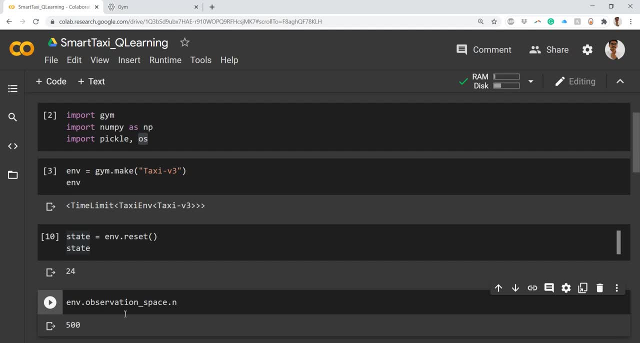 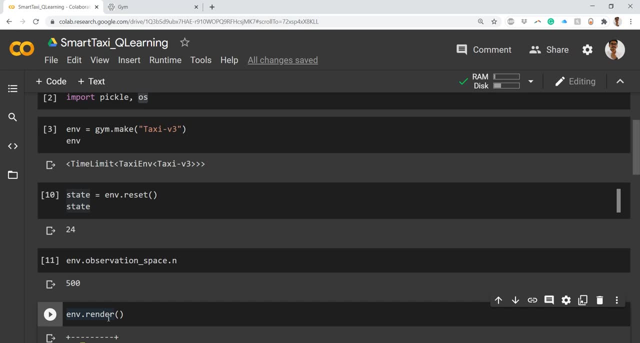 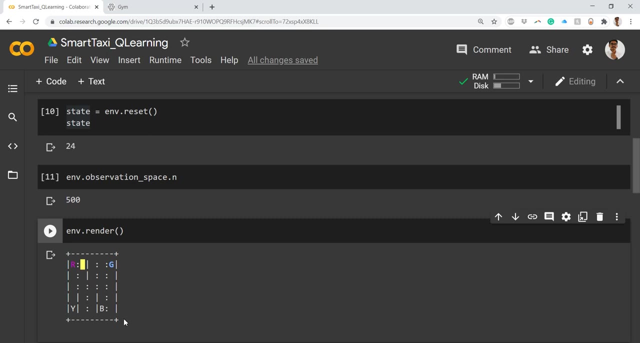 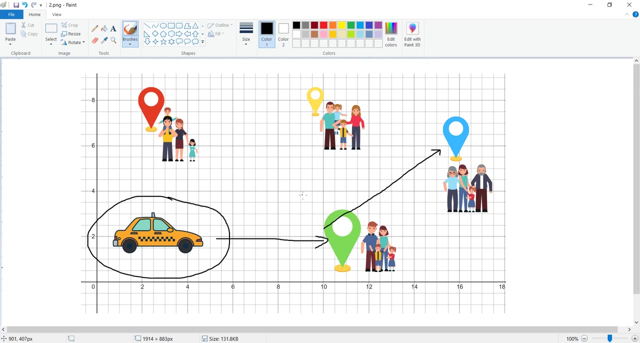 there are in total 500 observations in this particular environment and we just call the render method. so render method is used to just render the graphics. so this is how the graphics, or visualization, looks like in reinforcement learning, so as we have seen here. so this is diagram which is drawn by me just for a demonstration now here. 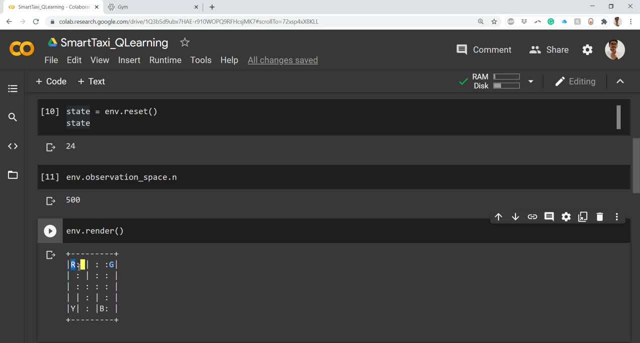 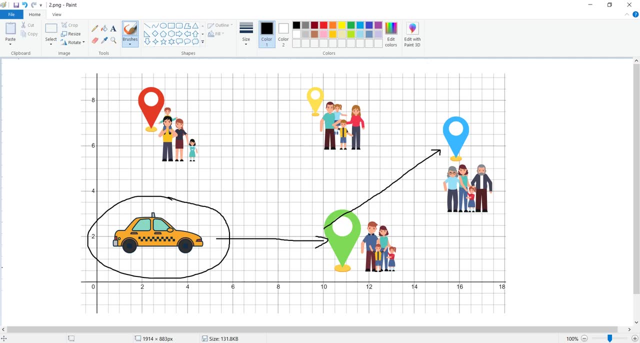 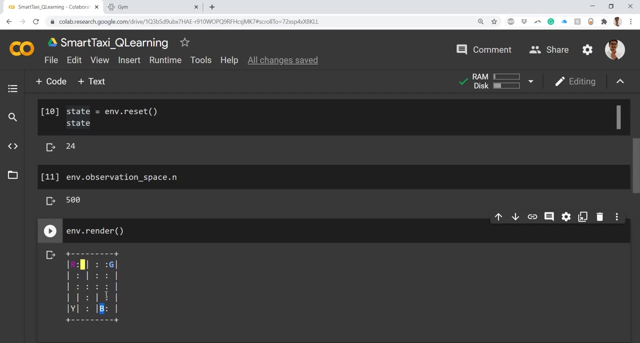 internally you have a red location that is here. then you have a location G that is green, Y and blue. so it corresponds to something like this and you can see as a demonstration of a game you have this kind of thing. so this is in two dimension how it basically looks like, so what you basically can see here, if you. 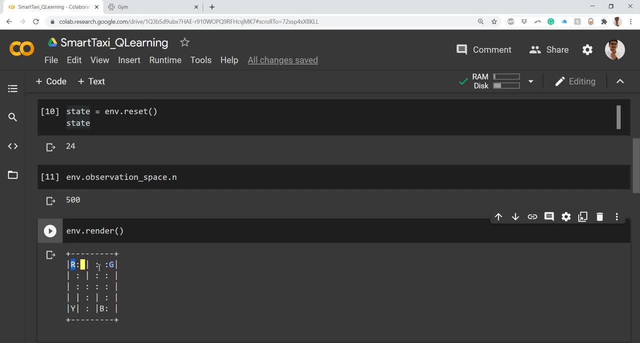 look here closely. this R and G- both are just highlighted- means from one location you have to pick the passenger and onto other location you have to drop them. so here, in this case, R is the pickup location and G is the drop location. now, if you ask me, how did I came to know this? 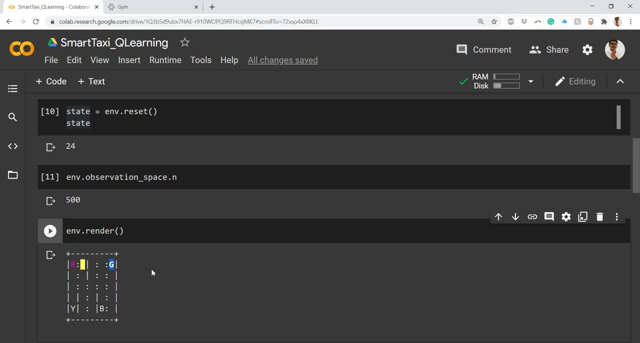 because I just read the source code. so from there these things are already predefined. so basically, this particular yellow thing which you can see here, this is nothing but your taxi. so the taxi can move in the left direction, right direction, top direction and bottom direction. so these many 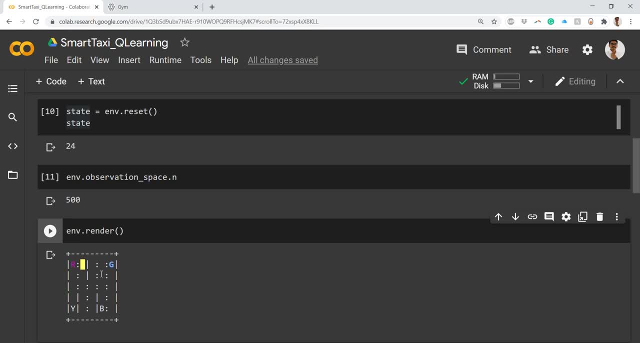 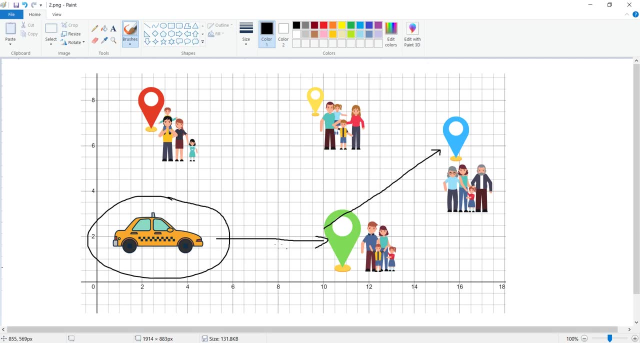 different actions are possible by the taxi and the additional actions are like pickup. so once the taxi is there at particular location, say, when we do the geographical calculation of this thing, what we observe, this: we get the latitude, longitude. so here, say, in this coordinate we have this taxi at location 2 to see, this is 1 example. so this particular taxi is at location 2. now if 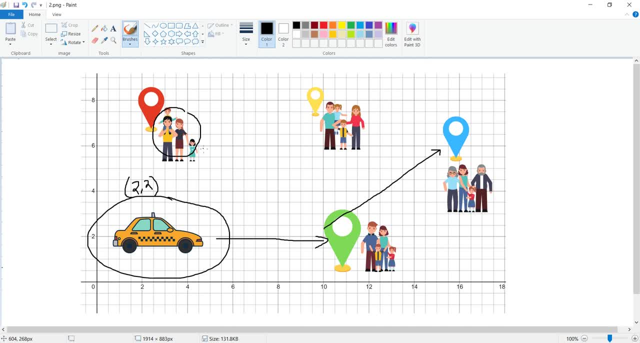 this passenger or these customers want to come with this level of skill, these human passengers, uh уждals extent leaded to say: this is where we are, why we get vacation. we get. if 75 الش queda still old is a much faster value. and all this, everything, body parts here. 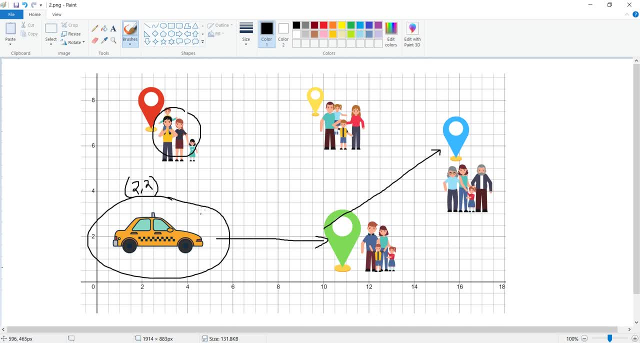 the axis of that smart taxi will access their coordinates. so say it is 4 comma 6. so first it has to make these many movements so that it will reach the particular location where the passenger is. so that's why we have this navigation. so that is in the top direction, left direction. 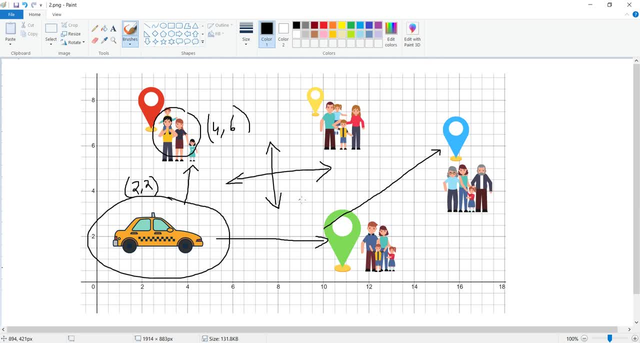 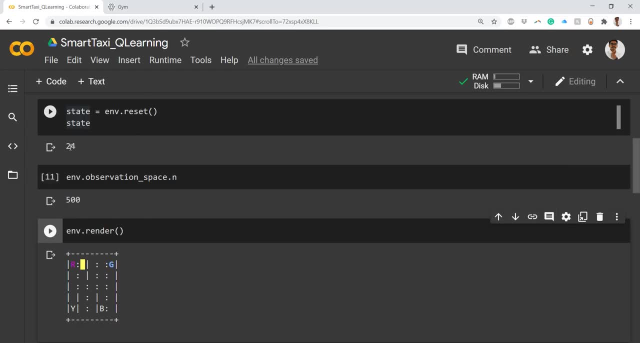 bottom direction and right direction. so these many navigations are possible in this particular 2d plane which you see. so here, what we see is it will first move to the left hand side, then it will take the passenger, and then it will do some right movements and finally, 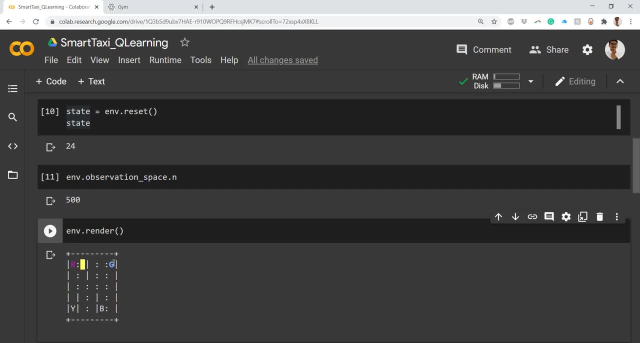 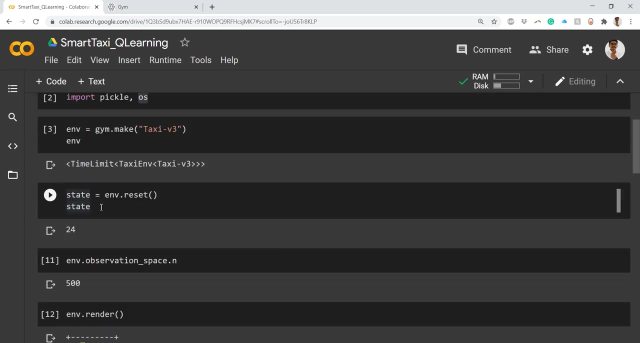 it will drop them off at the location, which is g. so this is how it looks. render is basically the same as the previous one, so it will take the passenger and then it will basically use to display the plot of that particular iteration or the environment, what you currently see. so we just look at the state. so we have currently 24 states. so that is. 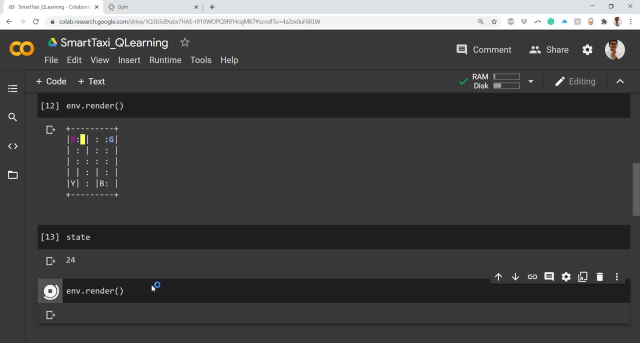 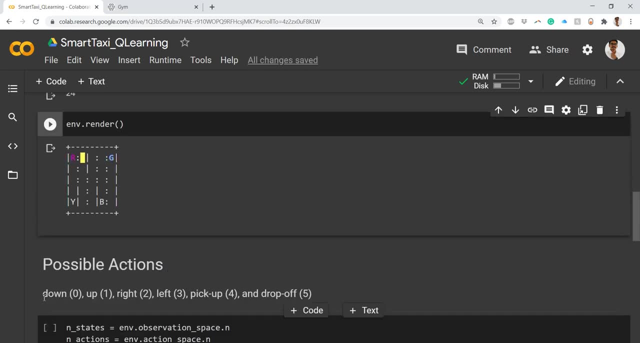 from here and we see the environment again. so that is the same thing which we see here. okay, so the possible actions which i said, that is down. so for down, we have a variable that is 0. for up, we have 1, right, 2, left, 3, pick up 4 and drop 5. 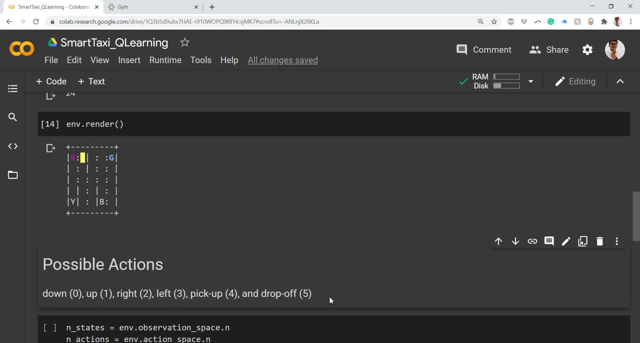 so this you can think of, like, say in your mobile phone, if you want to assign a caller tune. so they'll basically say like: for this song you have to press 1, for the next song you have to press 2, for the third song you have to press 3. so for this song you have to press 1, for the next song you have to press 2. 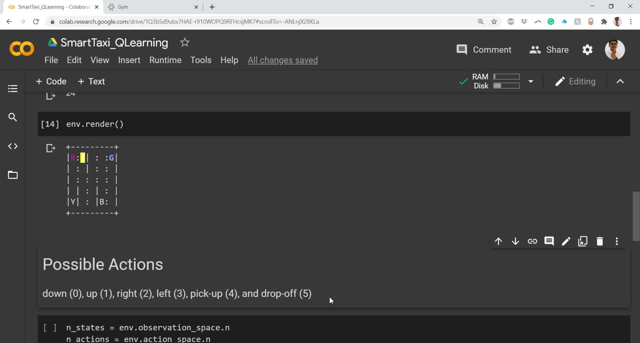 for every action it is mapped to one particular variable or a number so that it can be easily accessed or the movement can be easily done. so even in games. also, if you play different games using joysticks or the keyboard of your computer or laptop, you can have this different kinds of. 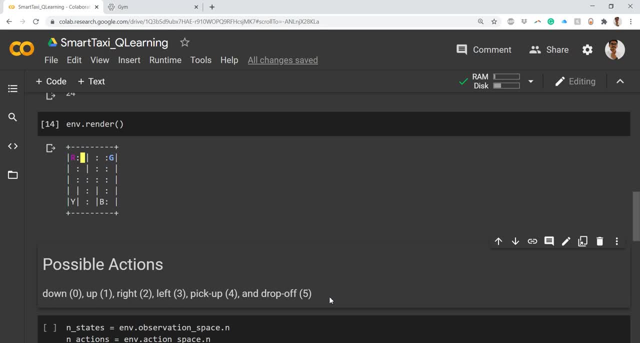 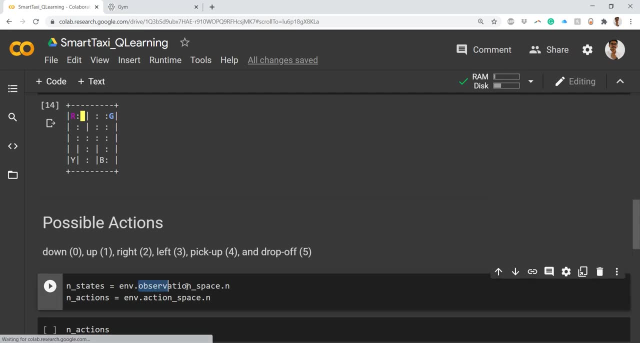 navigations. so these are the possible actions in that particular environment by which you can make different actions. so this is the possible actions in that particular environment by which you can make different moves. so the number of states from the observation underscore space dot n. so this is the environment variable that is present. so you have to call this variable in this. 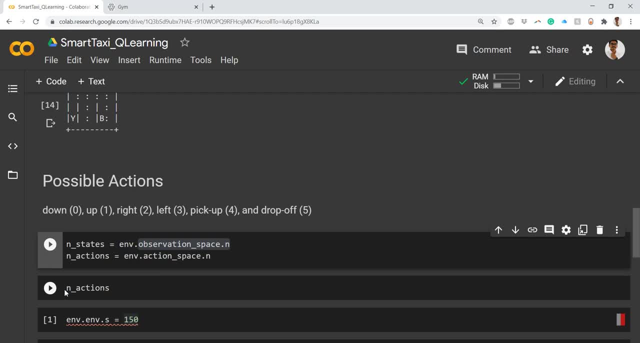 way only, so it will print the states and the actions. so i'll just print the actions. so we have 6 actions. so down 0, up 1, right 2, left 3, pick up 4 and drop 5. so you have 0 to 5, that is 6 actions. 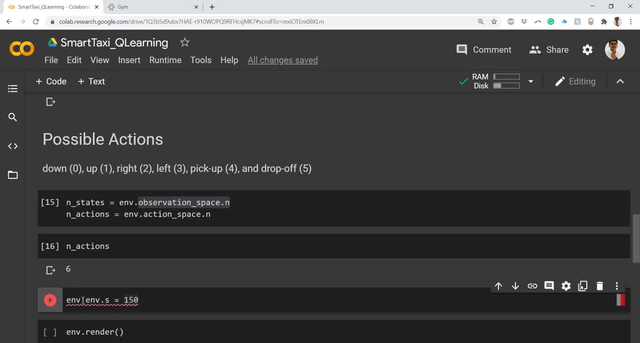 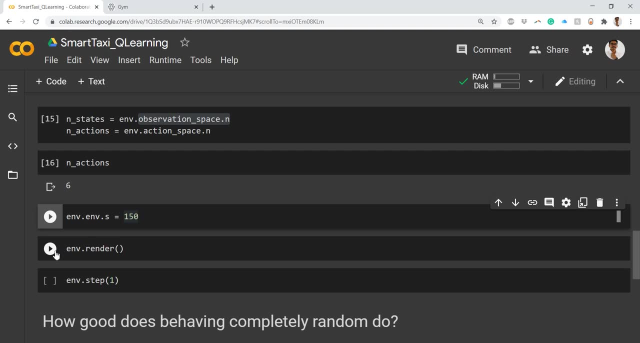 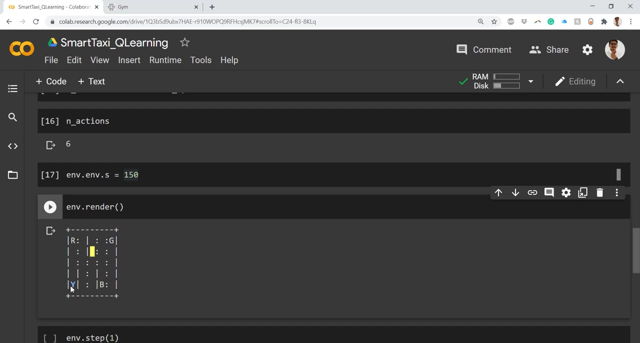 and this is the environment that i'm pre-setting to 150, and this is the render again. so what you saw here, that is the same thing that now what we are doing is i'm just changing the pickup location from y and the thing which you see here is the pick up location from y and the thing which you see here, 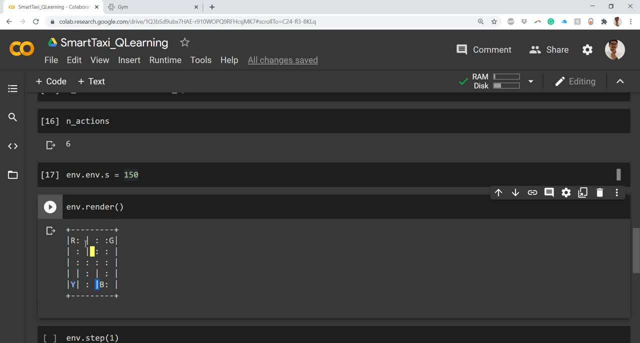 that is this: things, this are the barriers. so this can be considered as like some walls or some concrete walls which are present, from where you cannot go through. so you have to make some movements, either in the top direction, bottom, left, right, and then you can reach to that particular. 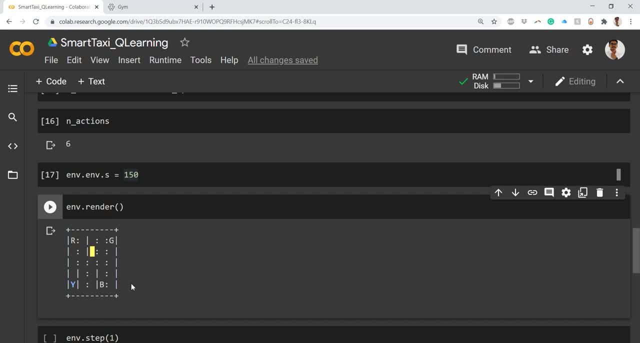 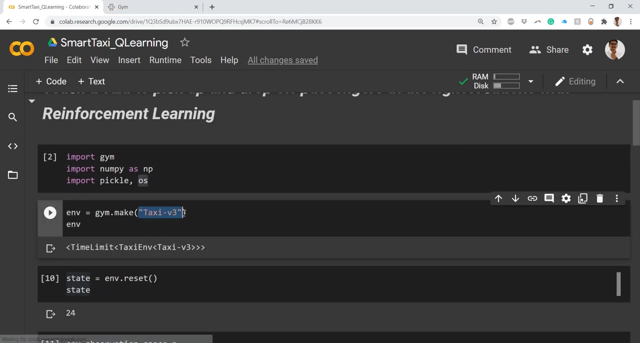 location where the passenger actually is. so that is the basic constraint that we are putting into this, else it will be a very simple example. so all these things are defined inside the environment variable. so when we just imported this particular thing, so in taxi v3 this kind of environment setting is already present. we are 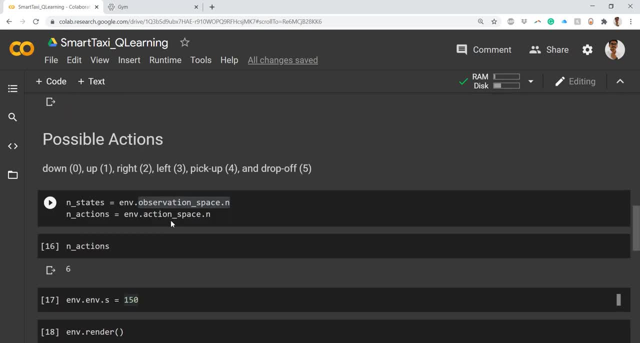 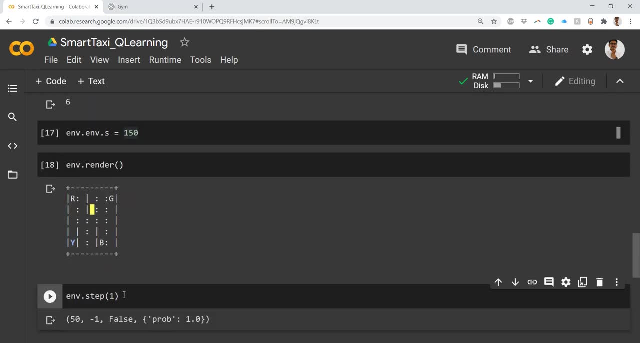 just doing the navigation and we are just trying to implement how it actually looks like. okay, so step is one particular method which will give the probability of reaching that state. so currently it is a one probability. probability of one means passenger is there inside the cab and zero probability means passenger is not there inside the cab and there are some other variables. 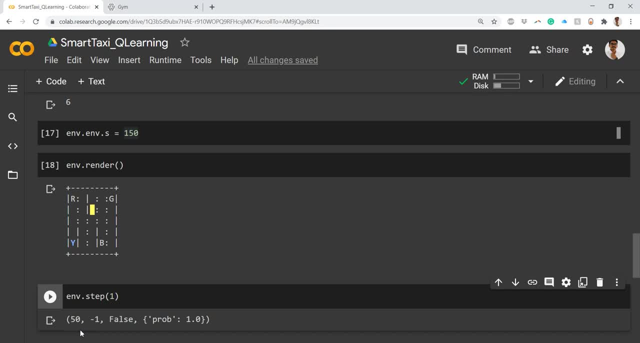 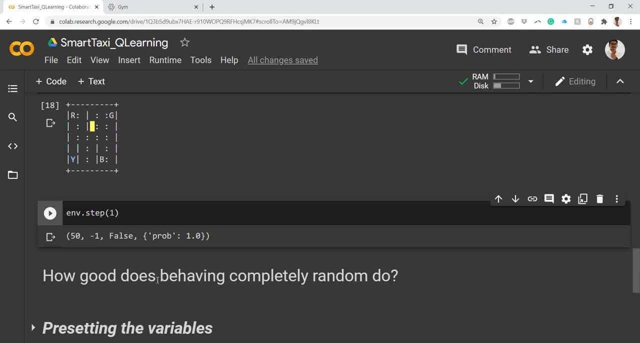 which is falls and 50 that will see subsequently when we do this. so now what we want to do is we want to look how this particular scenario is currently functional, to see if there is any kind of specification related to investigations. let's go on to the flipchart and see how it works. okay, so 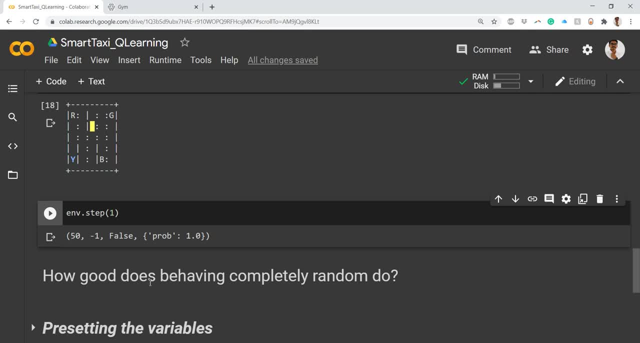 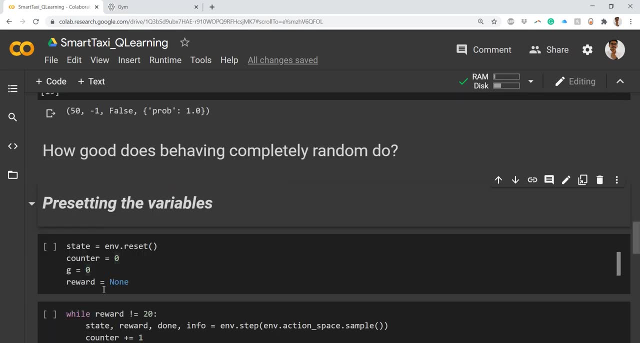 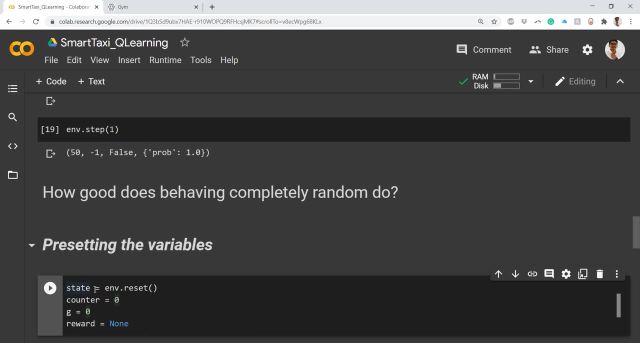 behaves when it is done in a random way. so for that we have to again preset the variables. so first I reset the state, so I call by dot reset, then I have the counter. so counter is another variable which is initialized to 0 for counting how many directions that particular taxi has made, and then G- G stands for my. 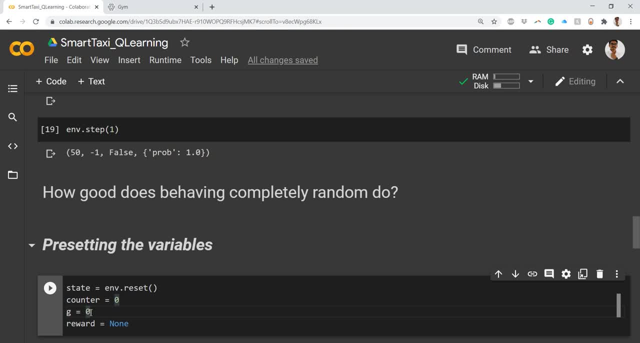 goal state whether the agent was successful in dropping the passenger at the correct location. so here it is 0, else it will be changed with some other variables, with some negative variables, negative rewards, which are there and here the reward? currently it is none, because initially so this is a boolean variable that we are passing. so that is. 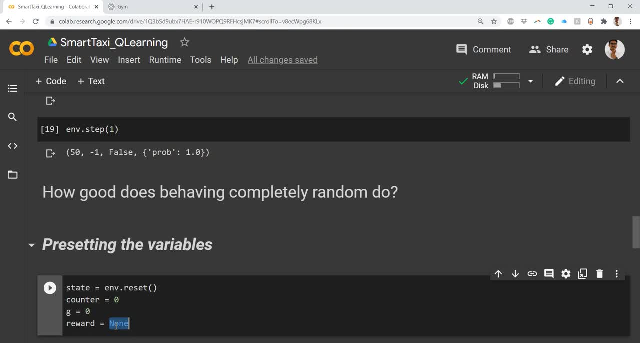 false or true. so if it is successful in picking up the location from where the user is or the passenger is, that will be a true, and when it will drop off the passenger, that particular location again it will be true. else, in case of driving the passenger between the paths, this will be false. so false means the cab and the passenger. 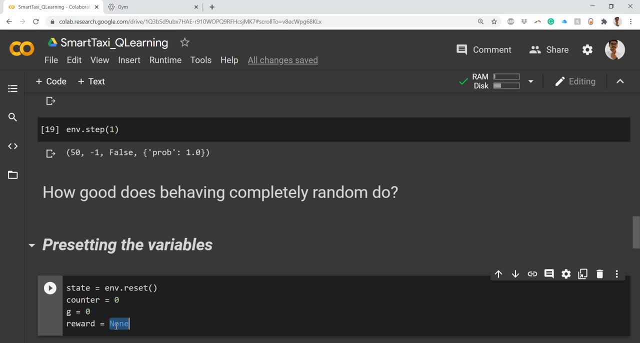 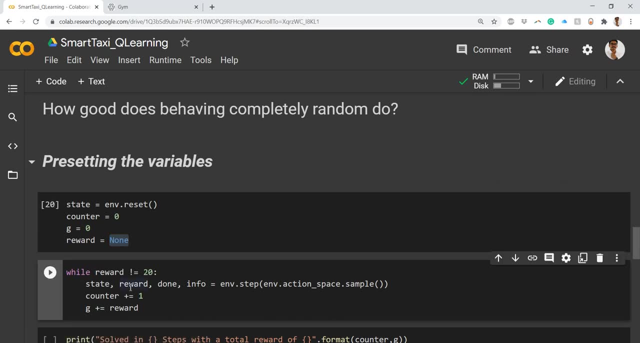 contained the cab are currently in a state of motion. ok, so now what we do is we'll just run a while loop. so inside this while loop we have certain rewards. so reward is nothing but where the passenger has successfully got into the cab and they have reached their destination. so if that is the case, 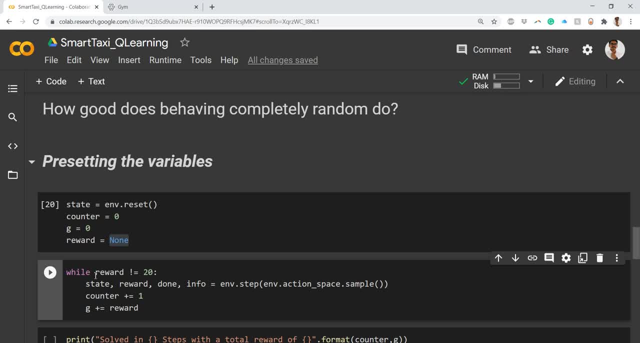 means the agent is successful in picking up the passenger from the source A, and if it has just drop them off at the correct location, then we'll assign a reward as 20. so 20 is the highest reward that is possible in this particular scenario. so here what we are doing is we are writing while reward not equal to 20. 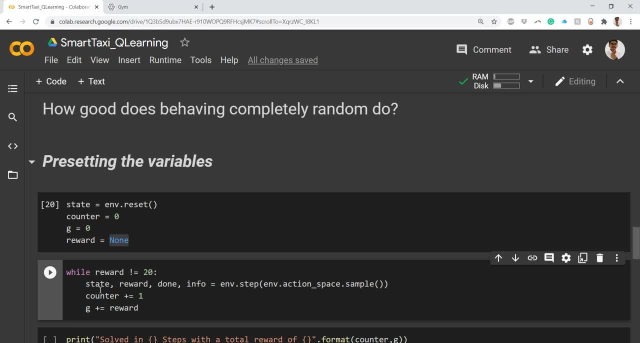 means. if that is not the case, then we want to initialize these many variables, that is, state, reward, done and info. so these are some kind of variables which are present inside the step function. so step function will need to perform the action. so what step function does is it will perform all the. 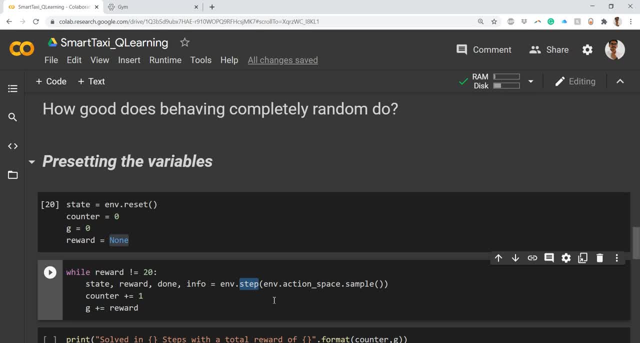 action at each step. so at each step it will move into one state. so from whenever you do the transition, it is from one state to another state. so that kind of single movements is possible with the help of state. and at the at every particular state you have a reward. so when you reach from state s to state st or st plus 1, you 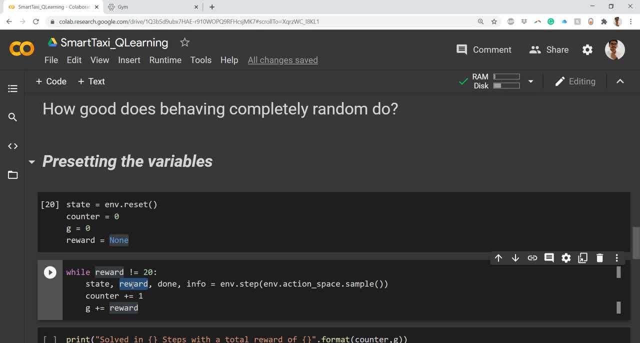 get a reward. it can be positive reward, can be negative reward, so it depends how the movement of the agent is done. so there that place, you get the reward, some remuneration, so that is nothing but your reward. and then done then can be true only in two possible states: when it is there at the pickup location or it is. 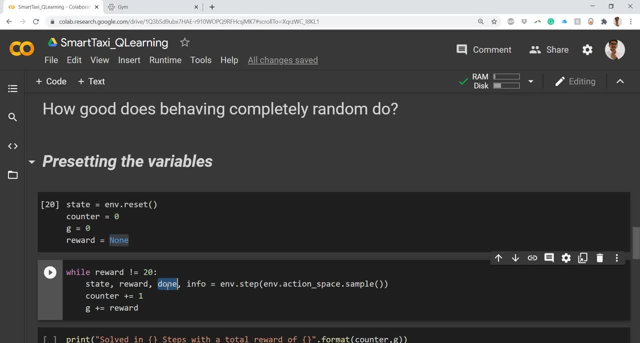 successful in picking up the passenger. so there the done value is true, and when it has dropped off at the correct location, integrated by the passenger, then it can be true. else, in all other scenarios or all at time places, this is to be false and the information, the current state of the 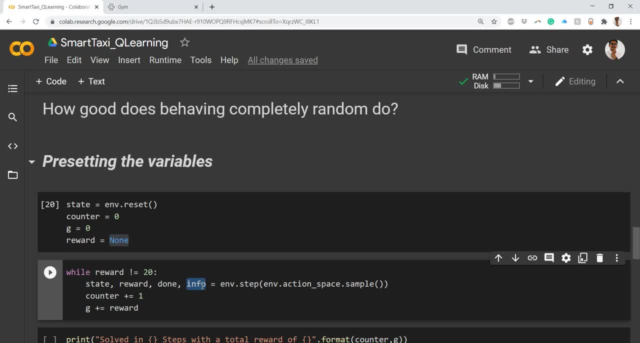 taxi or the smart taxi where it is at particular location. so that is the information, and we are just encoding these, everything into step function. so this is nothing but the packing that we already know from the basics, and then we are initializing the counter, every time by one. 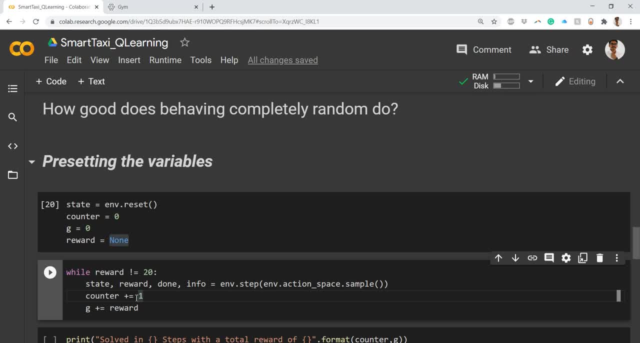 so we will do g plus reward. so we start initially with 0, then you accumulate with the reward and then after some particular time period or after some iterations, or after some episodes- we have to use the word episode in this reinforcement learning- then you'll reach your goal state. so that signifies this: 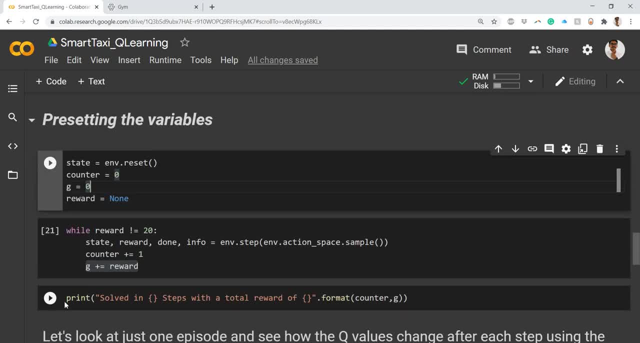 particular statement, then what we do is we just print how many steps are taken and with a total of how many rewards. so this particular syntax you are very much familiar. so this also we have discussed in the basics video. this is nothing but the replacement operator. so you know this kind of things are very much useful. 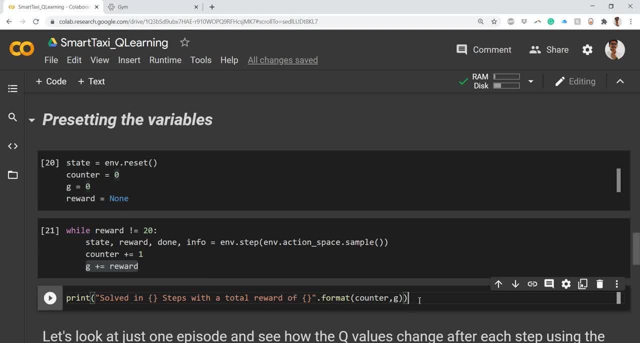 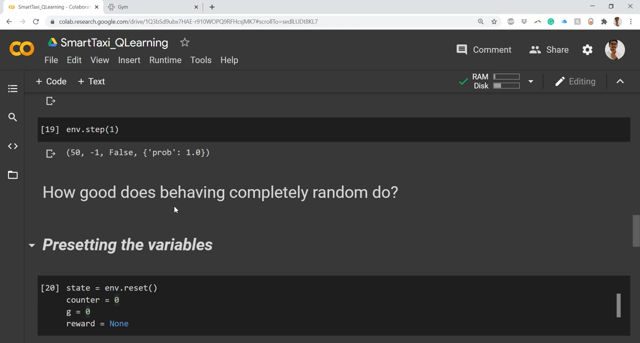 not only in the speech to text conversion, also in reinforcement learning scenarios where we use in small places. so we just format with the counter and the G so the counter variable, so I'll just print this, so this particular agent. now this is in a random setup, so we are making the agent behave in a completely 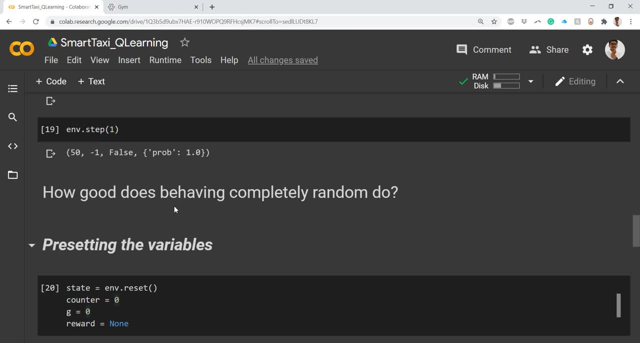 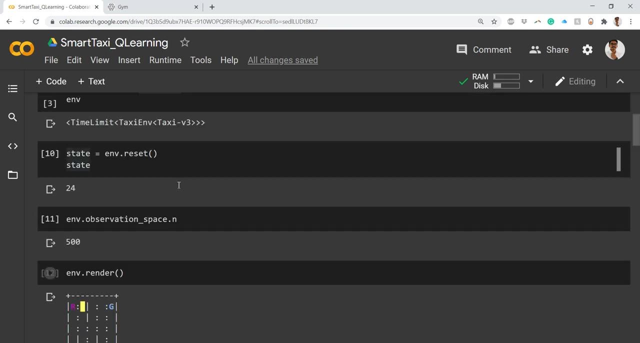 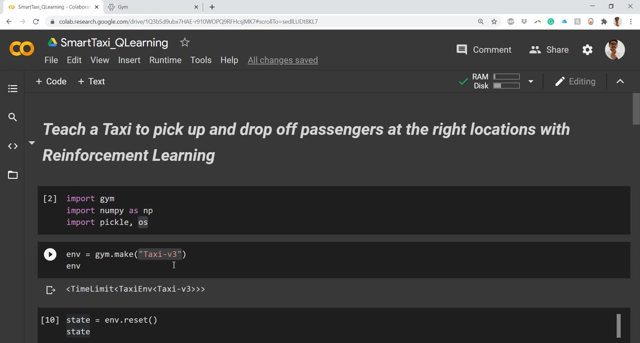 random way, so there was no hard code, algorithm or steps we were trying to incorporate into this. we can do that, but for that we have to make changes in the environment, since that control is not in our hand, since we are using this taxi v3. so, whoever is the developer, they have made the changes in this and 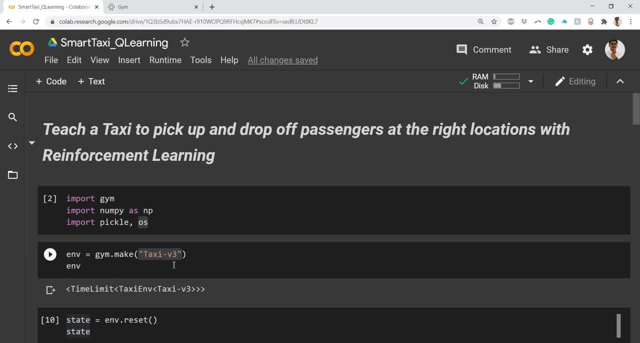 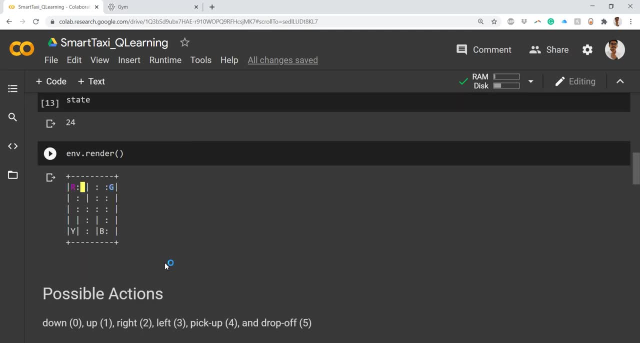 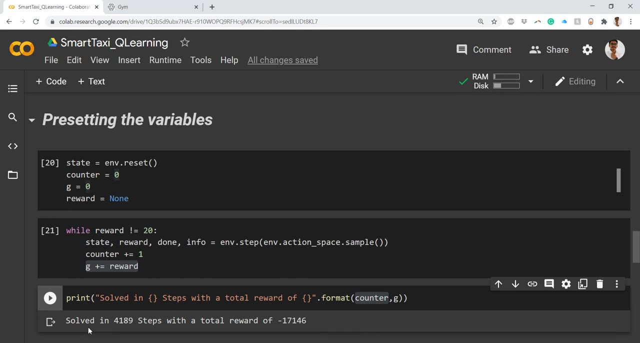 so, since we are only liable to make this or we are only able to run this, we can't do anything with this. but since this is a random approach, with this, we have done. so. what we can infer from this result is that the agent solved in 4189 steps, with a total reward of minus 17146. so here, just if, 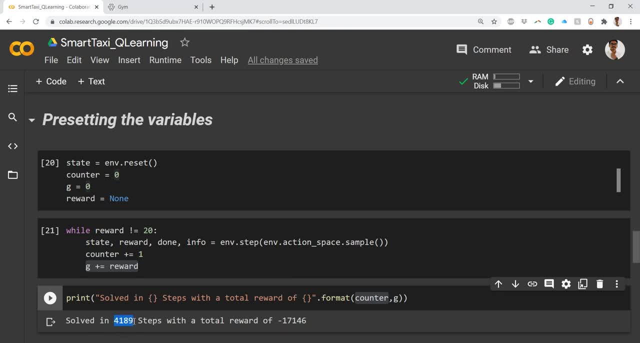 you know, the agent went for these many steps. so now these many steps- if a particular agent is doing means a randomized, self-driving autonomous car, if it is taking these many steps, so that steps is well done. so we can infer that the agent solved in 4189 steps, with a total reward of minus 17146. 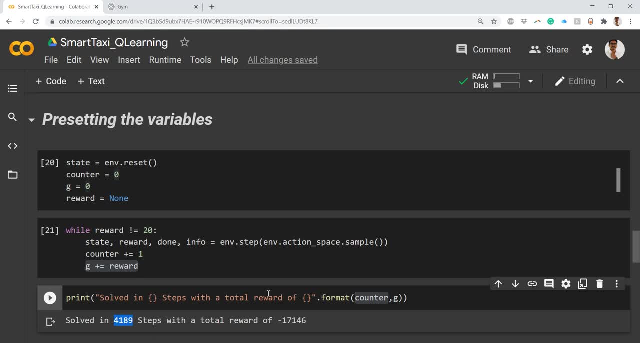 very high. so our goal is to, like the, minimize the steps and maximize the reward. so somewhere in between it is taking some incorrect paths. or the reward which it is getting, that is more over a negative reward as compared to positive reward, or the positive reward in between it has been. 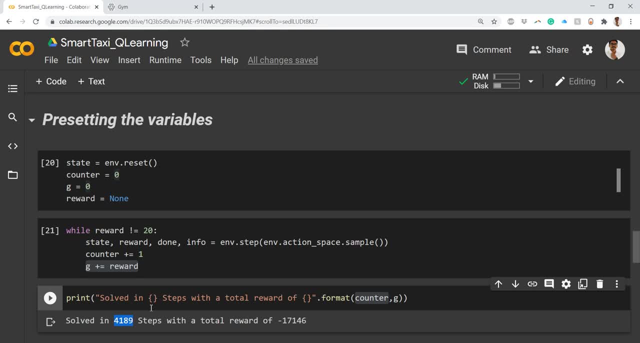 completely lost. that's why the reward is in the range of negative. so you have minus 17146. that is very bad. so obviously we should not be doing this. so we can infer that the agent. obviously we should not do anything in a random way. instead we have to define some steps, or in a 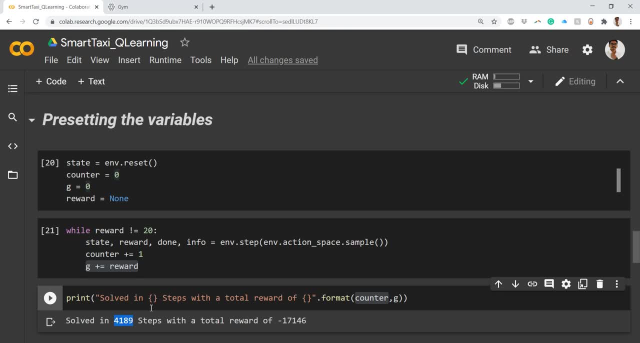 discipline manner so that we can reduce the number of steps and also we can maximize the reward. reward can be in smaller number, so we are not concerned about the digits- how many are there in the reward? but it should be something, but it should be positive. so minus 17000 is very bad. so 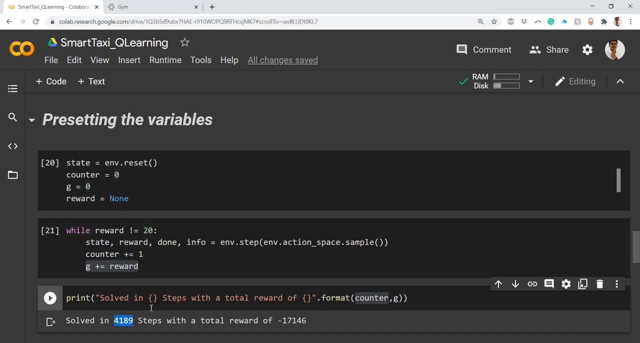 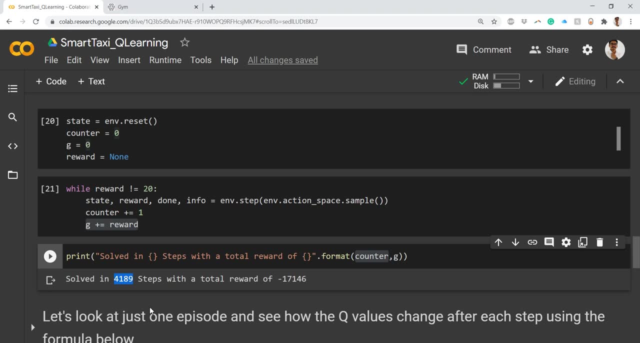 we don't want this, so we abolish this random approach in this particular scenario. so we then move forward and we now use the Q-learning, that is, quality learning that is at each step. we want to make use of the quality movement so that it will reach the destination with minimum. 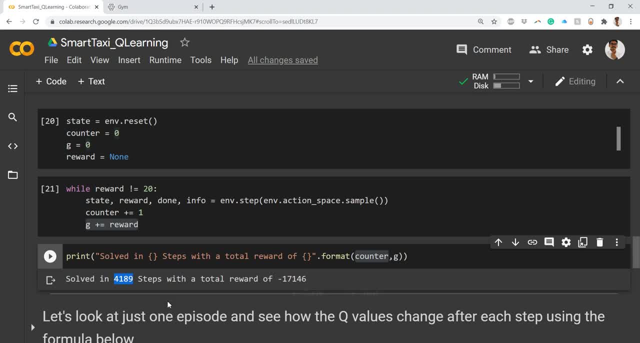 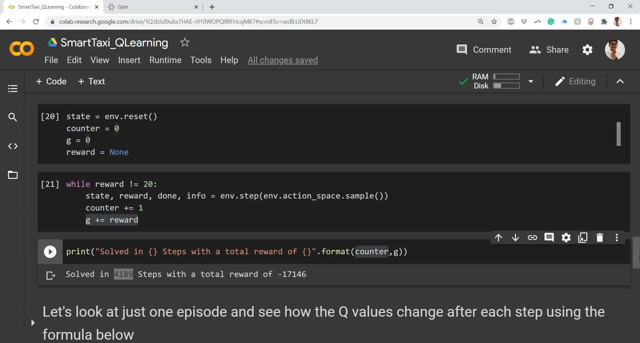 number of steps and with maximizing the reward. so now what we do is we just formulate just for one episode means what we areiez it m. Few episodes means we are doing the training for only once. so episode can be considered as your epoch in deep learning or in your machine learning, your training or the iteration. so these things in 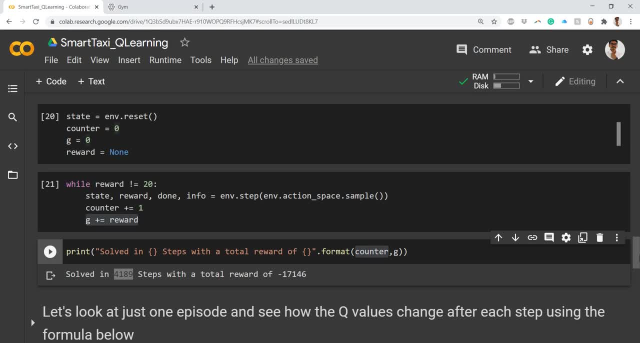 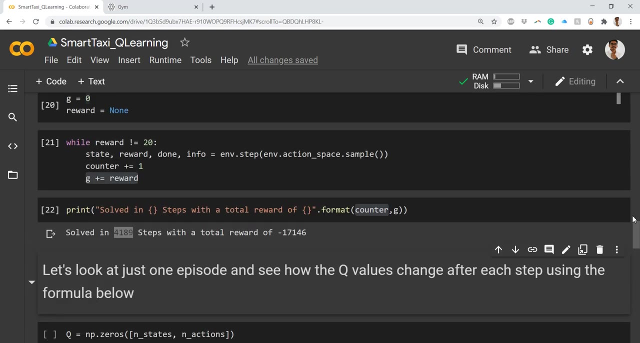 reinforcement learning. this terminology is called as episode, so for one episode we are training the agent and we'll see how the q value changes and we'll see how the math is done here. okay, so i'll just open this. so first, if you remember, in the q learning video i've discussed, you have 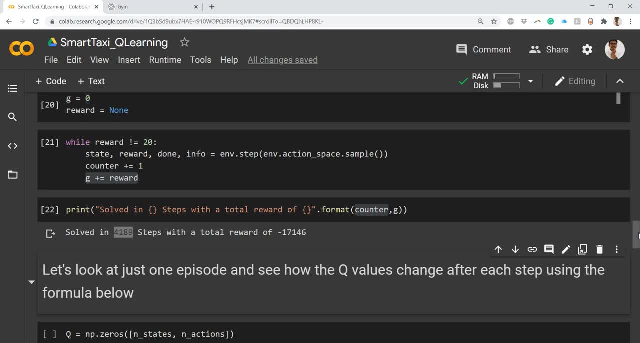 to initialize the q table. so you have two things: q table and q function. so q function is an extension of bellman equation. so that is completely mathematics. it depends upon the reward and the discount factor. but our q table will consist of all the possible states with all the possible actions. so all possible states, so that we got from here. 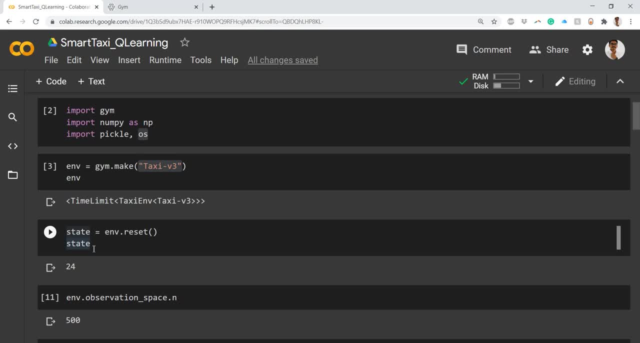 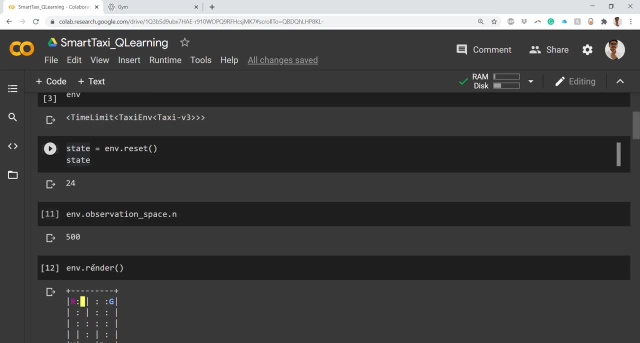 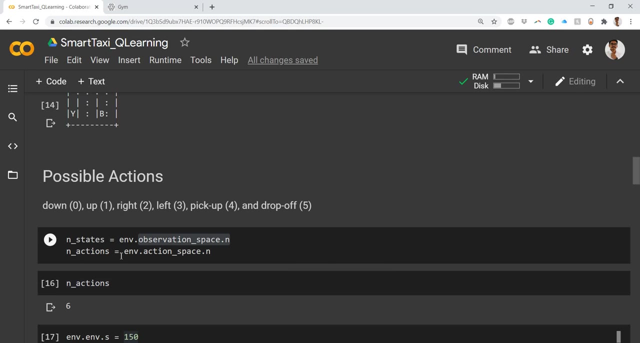 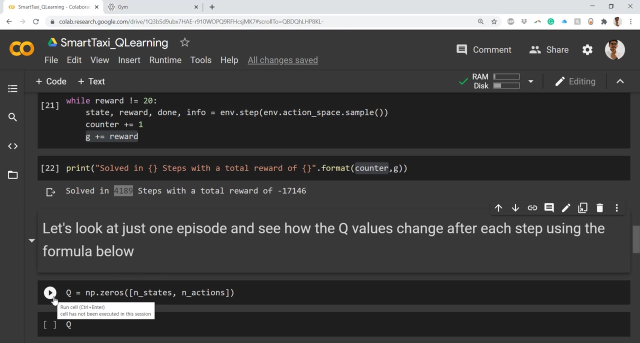 so state. this particular portion will correspond on the rows or it will reflect on the rows and on the columns. what you have is the actions. so whatever actions you get here, that is six different actions, these things. so these things makes your q table. so first you have to initialize the q with np, dot, zeros, so it will create an array. so you know about. 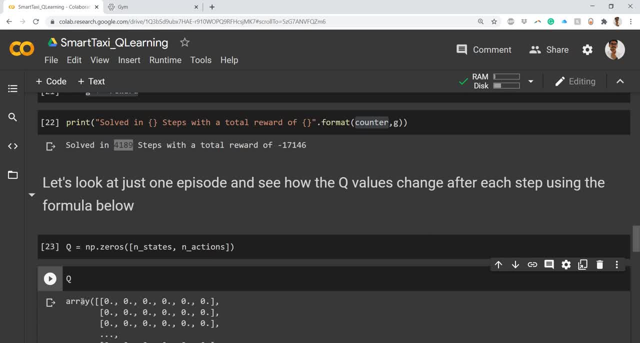 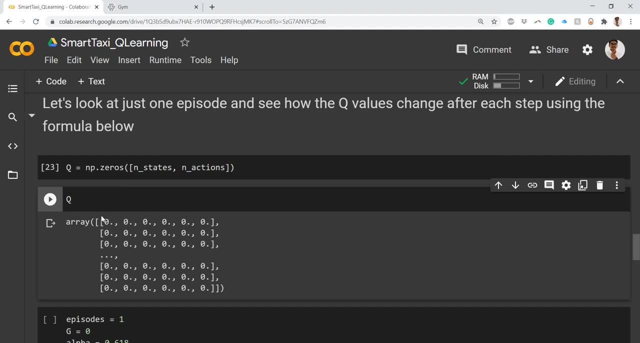 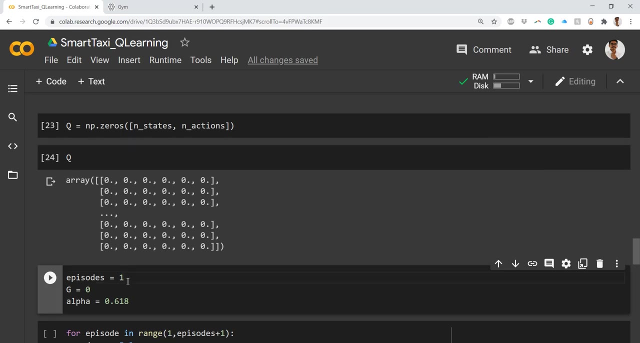 these things we have discussed in numpy arrays. so you can see it is a array of these many states and these many actions. okay, so now what we do is we just define the hyper parameters. so first is the episodes, so we are going to define the hyper parameters and we are going to define the 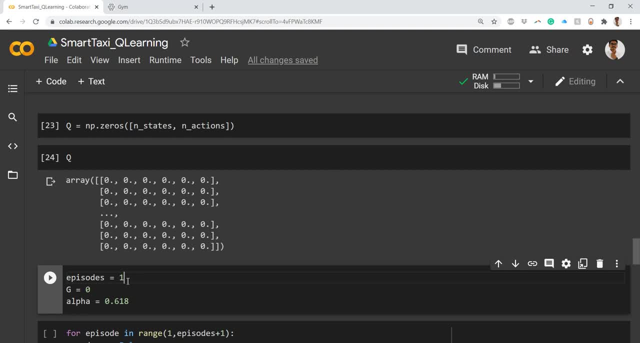 agent. so for how many episodes we want to make this agent train, or in how many episodes will this agent learn the particular environment? so here we are just putting one. let us see how this can be improved over the time period. and then we have g, that is goal state, that is, g is equal to zero. 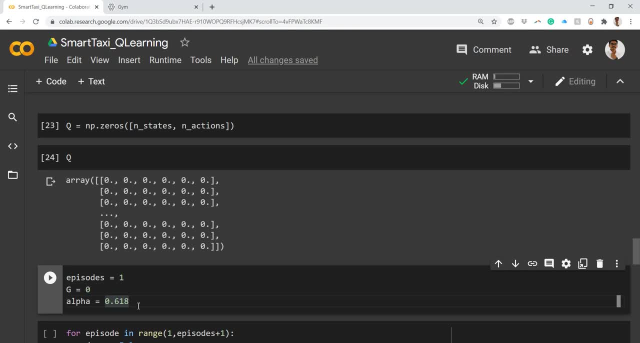 alpha is the learning parameter or the learning rate. that is again a hyper parameter that we are introducing here. we are putting the value zero to one and we are putting the value zero to one and six- eight. that is completely random. it's upon you. you can change this and tweak the parameters. 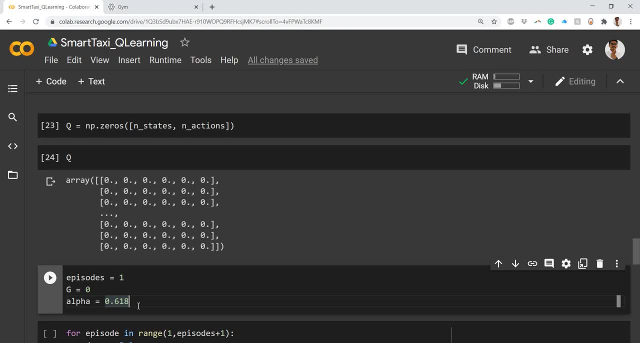 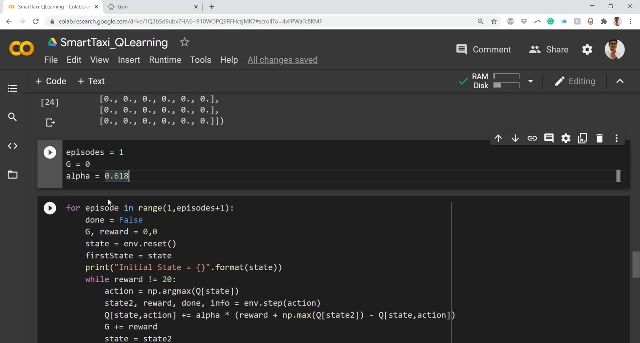 and change and see how it will affect the agent in reaching the final goal state, and also the rewards, whether it's maximized or minimized. okay, so then we move forward and we just implement for loop, so for each episode in the range of one. so we are initially starting the episode from. 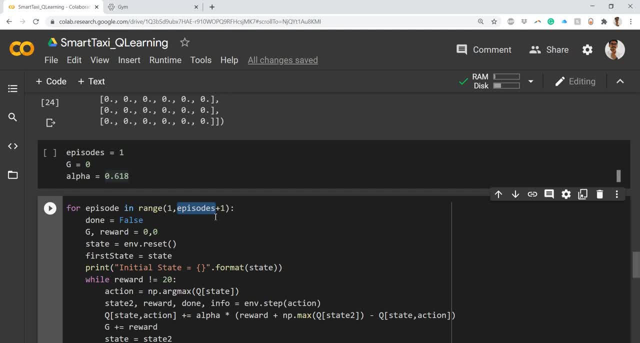 one and the number of episodes. so here, episodes, what we are doing is from one plus one, that is two. so it will just do only for one episode. then later we'll change this and we'll see how it is done. so we are just implementing for loop with the help of range, and done initially is false, so done is. 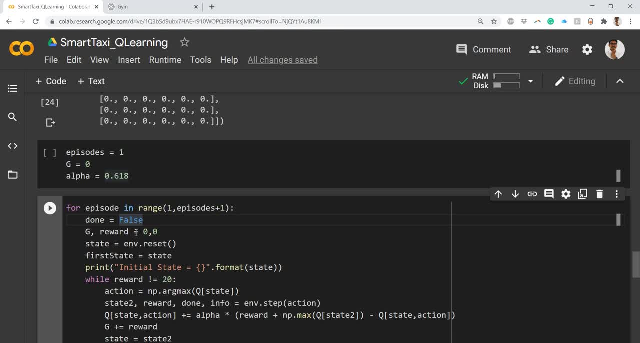 nothing but your final state value. so we are just implementing for loop with the help of range, and done initially is false, so done is nothing but your final state value, whether it has reached or not reached. okay, so whether the agent was successful in picking up the passenger and making them reach the final destination. so here, currently, we are making this. 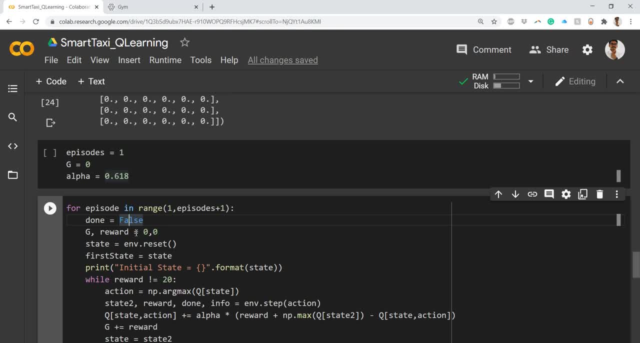 as false. later, when it reaches, or when it is successful in making the passenger reach at the final destination, then we'll change it to true the goal state and the reward- initially it is 0, 0. then what we do is we just reset the environment. whatever is there. so this kind of activity you 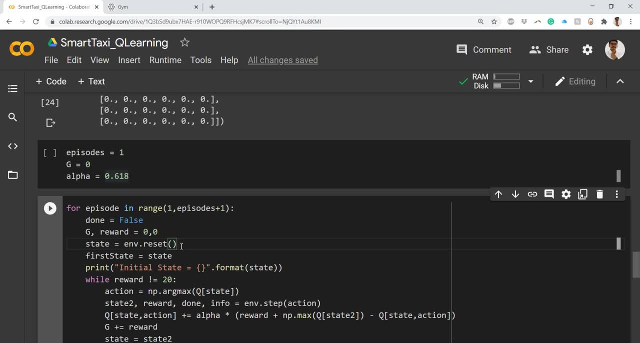 have to do whenever you do the new iteration every now and then, because sometimes the old iteration might be there in the system. so it will try to pick up the old environment variables and old environment states and then it will try to do learning on that. so that can cause a kind of 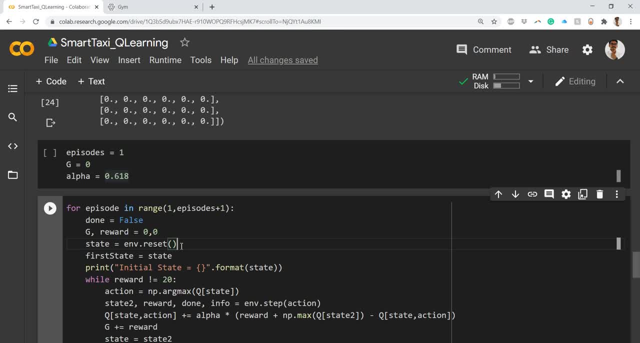 other deviation in learning your agent and when you will bond the product to your machine during the cycle, then it will really see it's done. that's why many times you cannot have all of them, because it is the only thing that's involved. so we don't take the link to์. 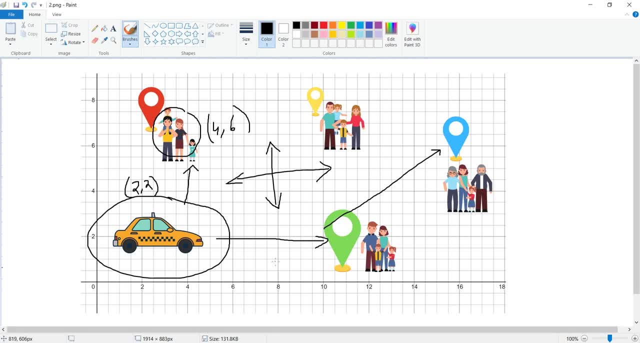 you guys set built. couldn't you let calm? this can be done right. 11, 11, 11, 11 Wave in your machine automatically. so this where you can use this at the local level. I do not use this, but we use in mobile mind, so we don't want done all those things to happen, so that's. 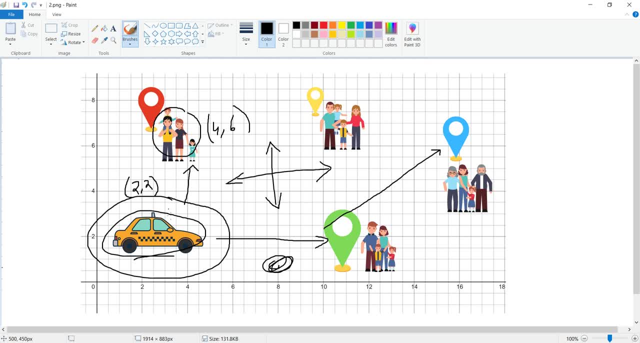 why we reset the environment, committed so it can be at any place. so it could be like it has picked this particular customer and it has made them reach here. So now, if you initialize this or if you call this taxi from this particular location, this will be its first state, as opposed to before. this was the first state. 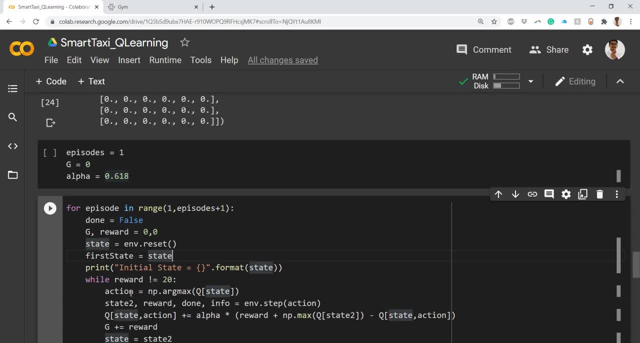 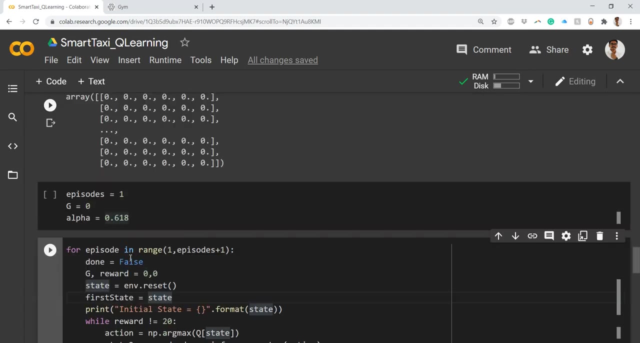 So for that we have to initialize the state to first state. then we'll just print what the initial state is or initial state was, and then we just implement the while loop. what is there here? So while reward: not equal to 20. if it is equal to 20, that means it has reached the goal state. 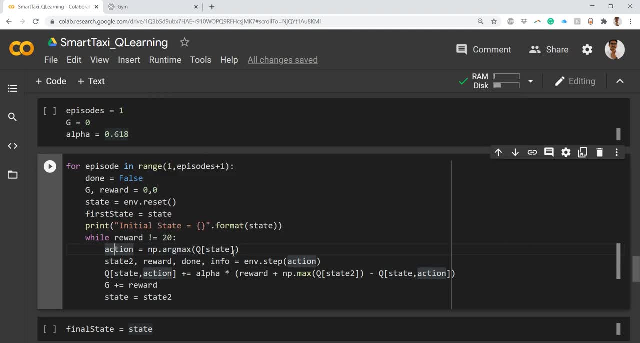 and the action that we want to do. that is dependent upon the state. so, dependent upon each of the state, it has to maximize the actions that it want to perform. Then we initialize a state to variable reward and done and info we just put into action. 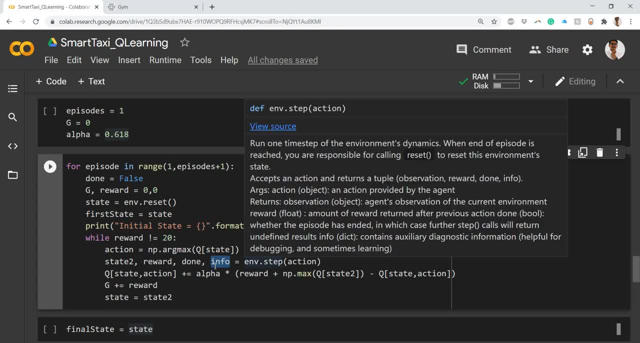 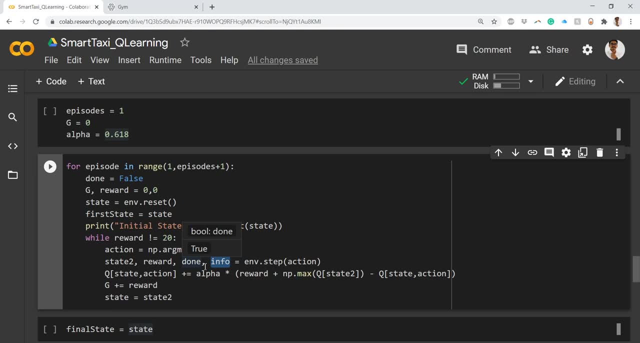 So the current action, that is from the first state, it will take the second step or the second state, then it will get the reward. then it will check whether it has reached the destination or not. So here it is false. if it is the destination, then it will be changed to true and the information. 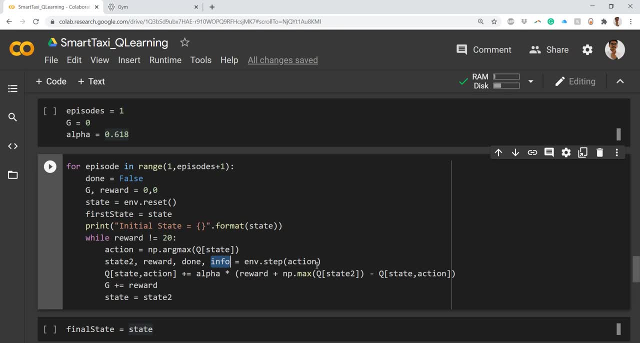 current status, So that agent that we have to encode in the action. So this particular thing which you see here highlighted, this is done at each step. So at one particular point of step this is executed. Then we do the Q learning, or Q learning, since you know it takes two parameters: or it's a 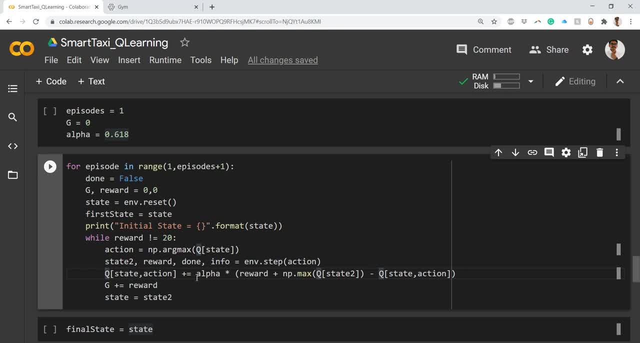 function of two things: state and action, S and A, and to this we add the same thing and again. so for that we have this plus equal to. so that means Q of state action is equal to Q of state action, plus we have the alpha, that is the learning rate, that is 0.618.. 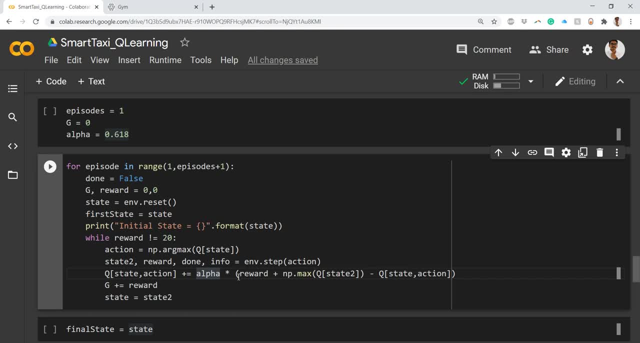 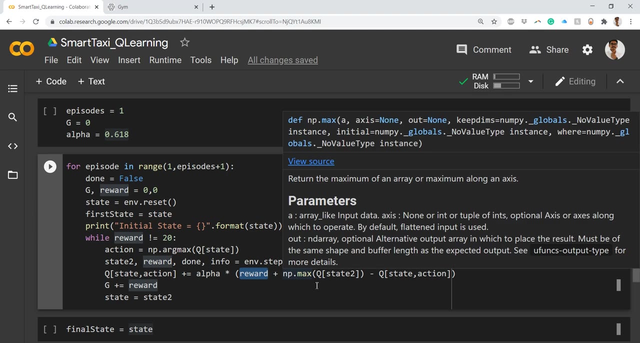 Then we multiply the entire thing with the block, So that block- if you remember from the video, the conceptual video of Q learning- we have the reward and with that reward we have added the max. That is nothing But your. So this is another function which is present in NumPy. 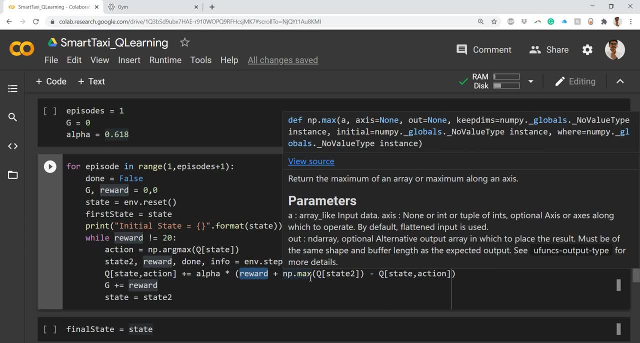 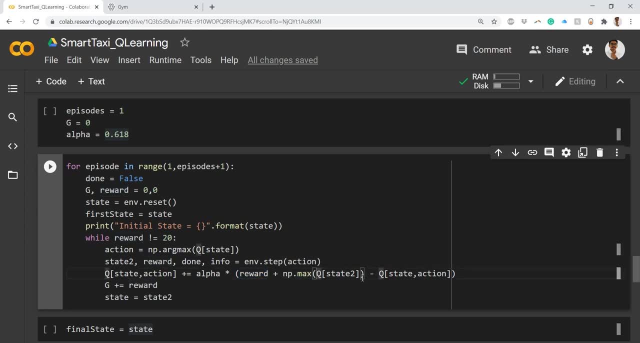 So it will maximize whatever value is there present inside that particular system. So in that you have your Q state to minus Q state and action. So this thing which you see on the right hand side, that is the older one and this thing is the current one, that is a new one. 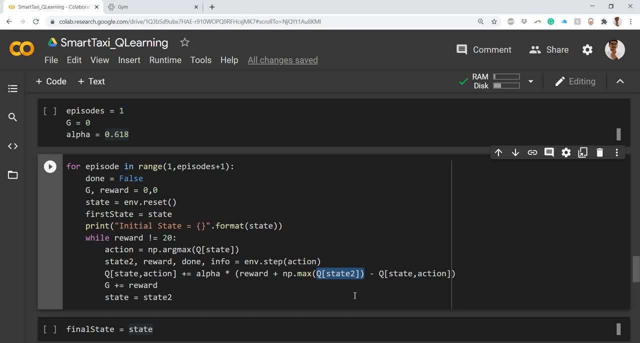 So if you want to have More details over this, you can watch the Q learning conceptual video there. I have discussed each and every bits and pieces of this thing in detail. Then, once you perform the Q learning here, then you have to update your reward. 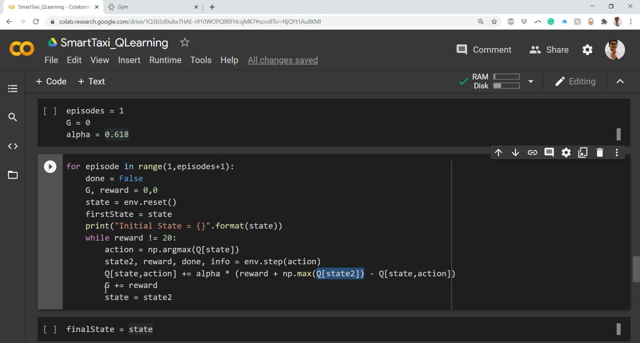 Once you reach the goal state, or whenever you are approaching the goal state, you have to accumulate the reward and maximize it, and then you initialize the state to as your state. So that's it. So now, whenever you are repeating this action again and again until you reach the reward, 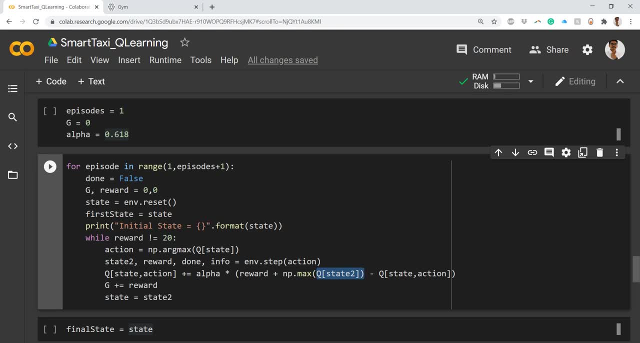 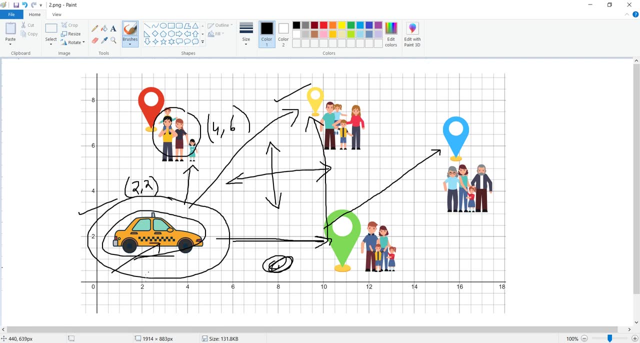 state you will be starting in that particular position. So just to make you understand, say it was at this part, or the agent taxi was at this particular location. then it moved to this particular location. So it had some kind of rewards, say a reward of five units. then it moved to this state. 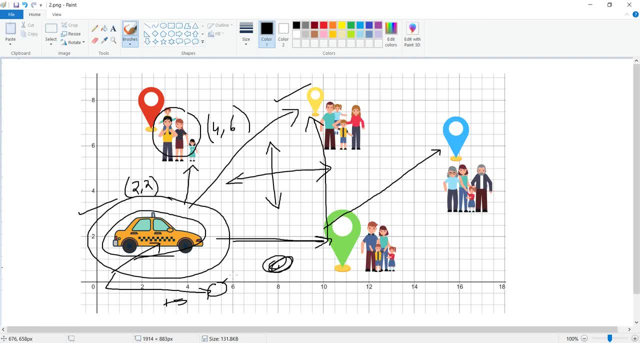 Now this state is the new state. from this state it will move to some other location. Now this location or the navigation is in this particular notation, that is, upward, downward, left and right. Then it will move to some location. It will probably have some reward. 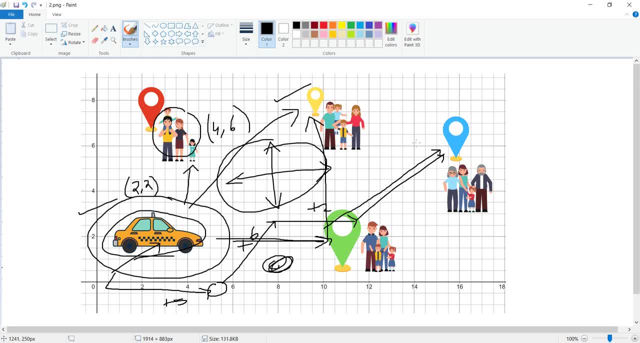 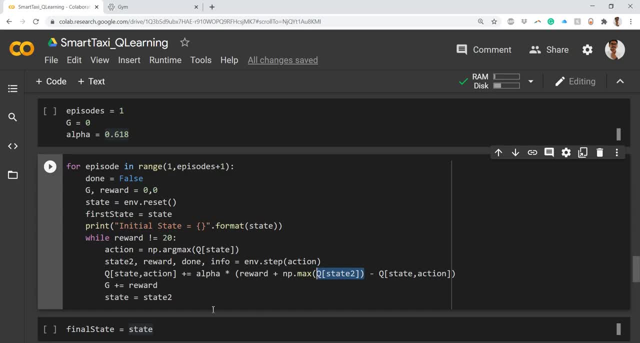 Say: here also, you have some reward and until it reaches the destination you will get the reward plus 20. And finally it will drop the passengers off at that particular location. So this is the new state At that particular location. So that is this entire block. what is doing will just run this okay. 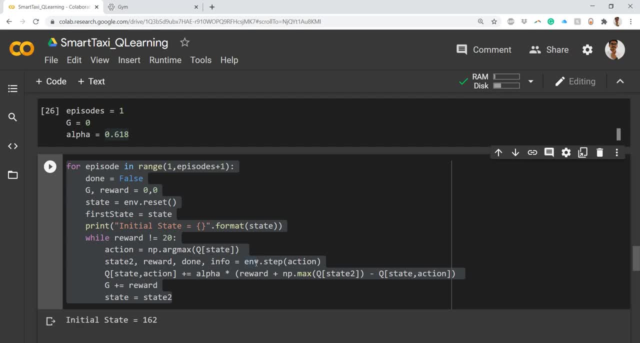 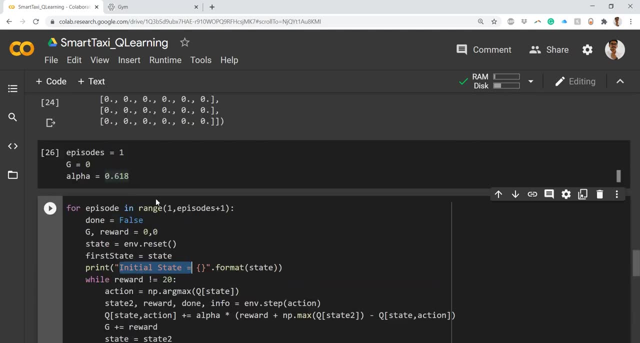 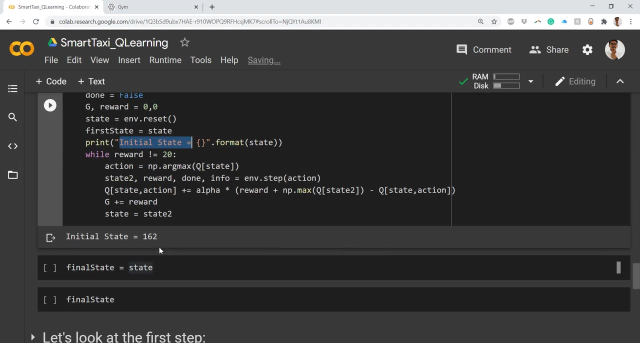 We have not run this, okay, So initial state here now it is 162, because we have just kept the episodes as one. So for one episode the initial state here it is saying it as 162.. Okay, So if it is completely random inside the environment how it is there, then the final. 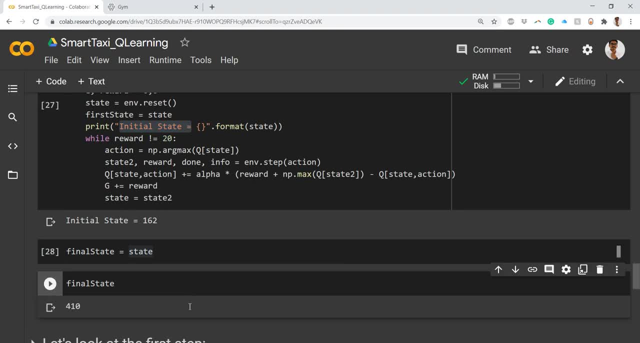 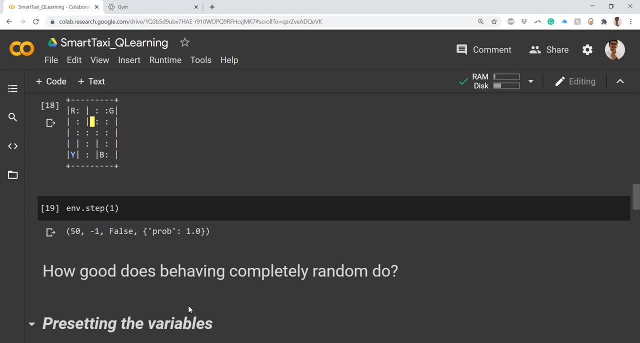 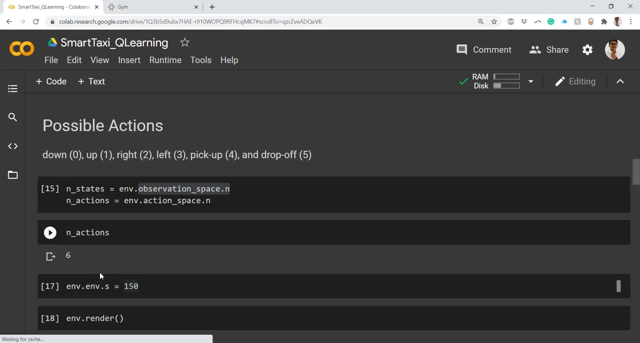 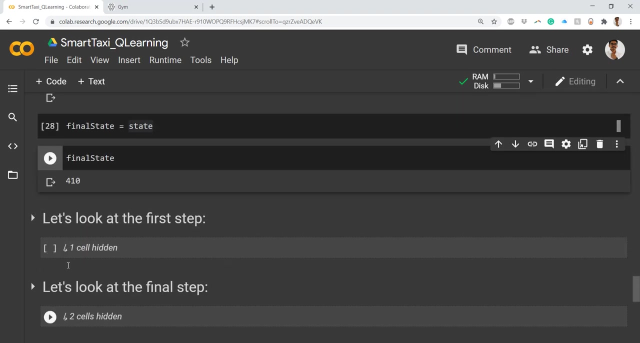 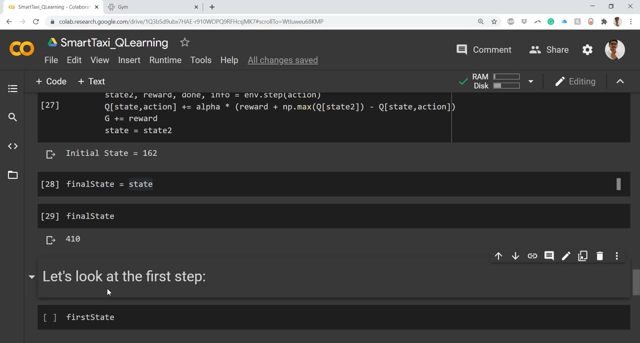 state. let us see what is the final state. So final state is 410. okay, So here let us see. here also, we had the final state. So this is a state, and, okay, we just have defined the state here. So now, since what we have done is we have trained our agent for only just one episode, 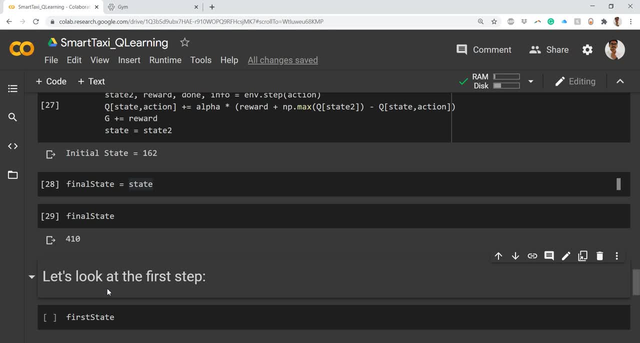 That is not enough. We have to train that particular agent for multiple episodes. So even if in the case of human beings also, whenever we are going to one particular strange location which we are not familiar, or to one particular location or to one particular city, 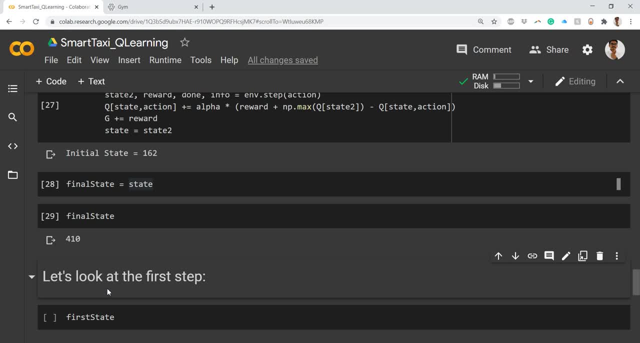 we have to do the training, Or we have to go to that location every now and then, or whenever we get time we have to visit that. So we do a long drive or short drive to that location so that it becomes easier, and also it becomes easier for us to understand what are the other possible alternatives, which 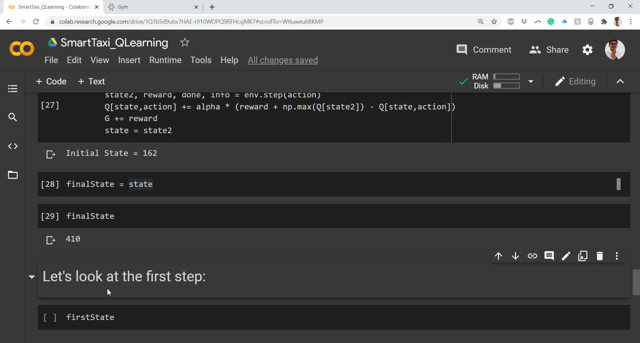 are there that particular pathway. So similar is the case. you have to teach the agent just with only one episode. it will not learn anything, Okay, So you have to make at least learn to 500 or 1000 episodes. that will see how the change. 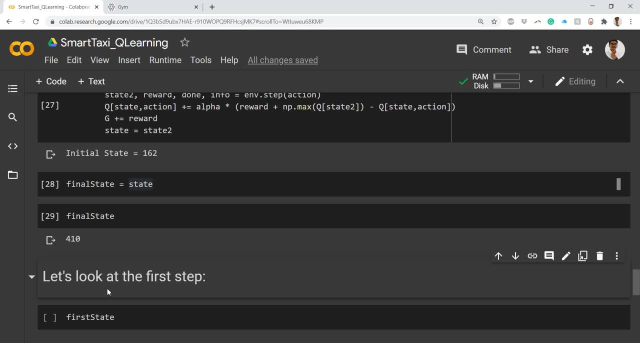 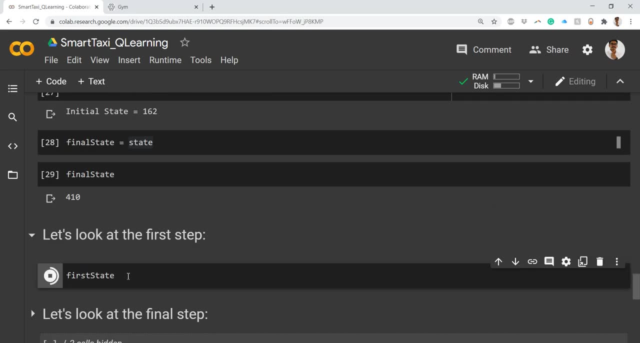 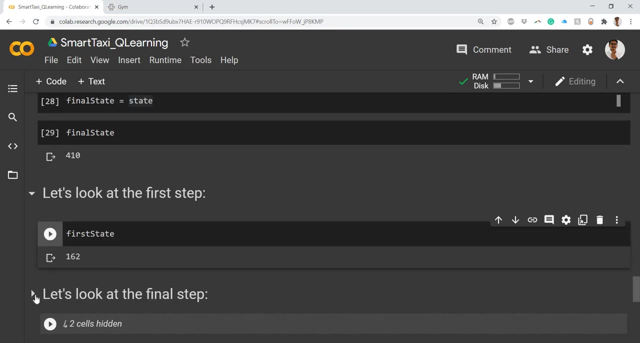 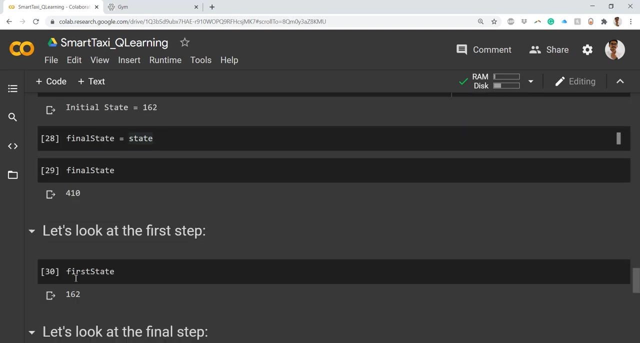 of episode will make the agent converse to that particular goal state, So it has a very powerful impact. Okay, So first we look at the first state. So here we are just implementing the algorithm again and again. So here we'll just look at the final state. 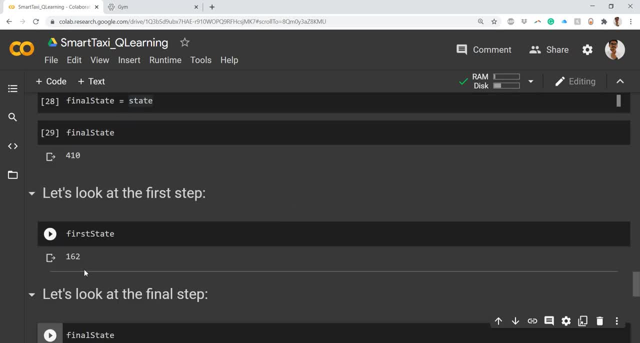 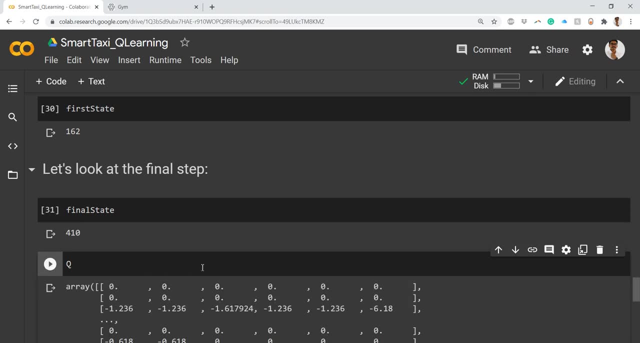 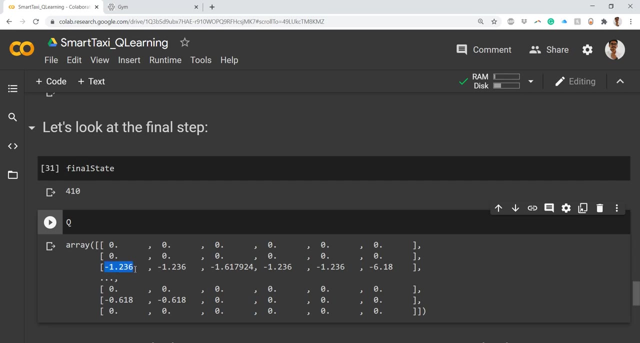 Okay, So here the final state is 410, first it is 162, final step is 410.. The Q table: how it basically looks after all the iterations calculations. it looks something like this: So wherever you see a negative values, though, that means you have some negative rewards. 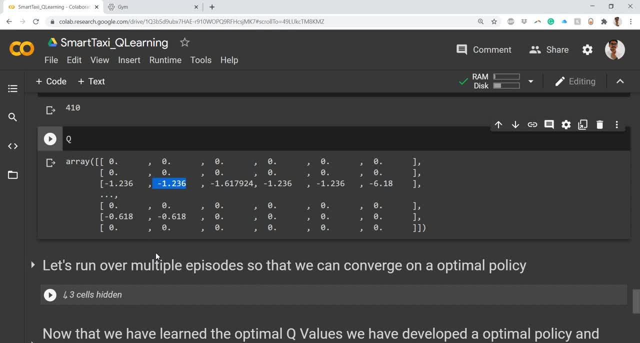 Okay, So now this was the illustration, Okay, Okay, Okay. So now let's go ahead and see what the impact of just having only one episode. Now we want to run over multiple episodes and let's see how we can convert to an optimal. 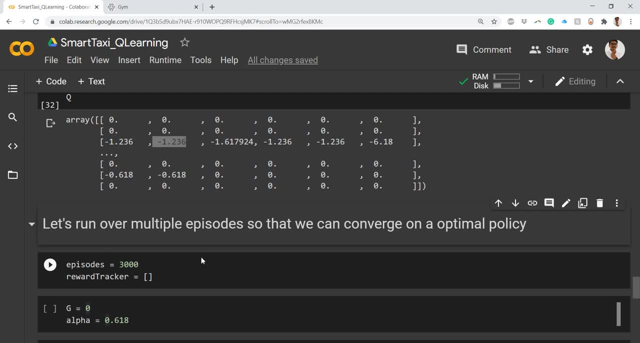 policy, or what is the optimal path in gaining the maximizing the rewards and also with minimal number of steps. So here, what we are doing is we are keeping the episodes for 3000.. Okay, So this is the result of the conversion, Okay. 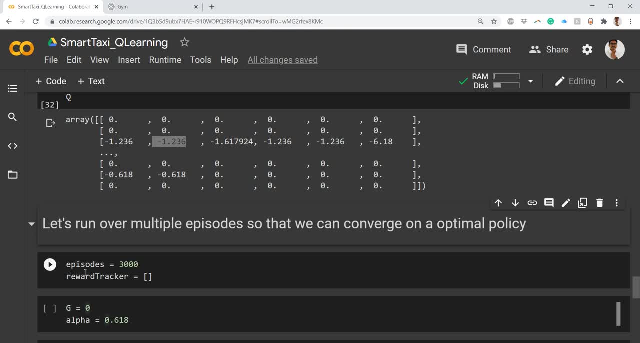 3000. so instead of one we have to now iterate it for 3000, so for 3000 episodes. it will learn that particular environment and it will try to improve how it can maximize the reward. and then you have a list. so in list i'm putting a reward tracker, so how much reward it has gained so far after it has. 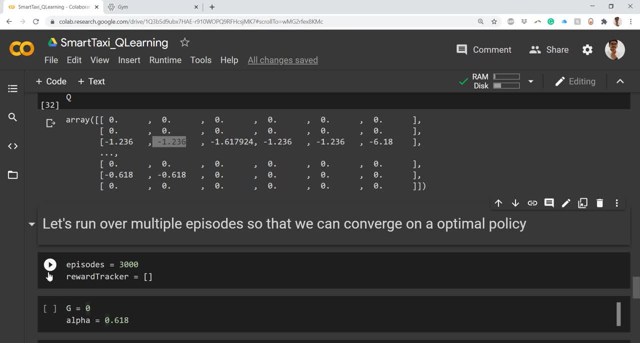 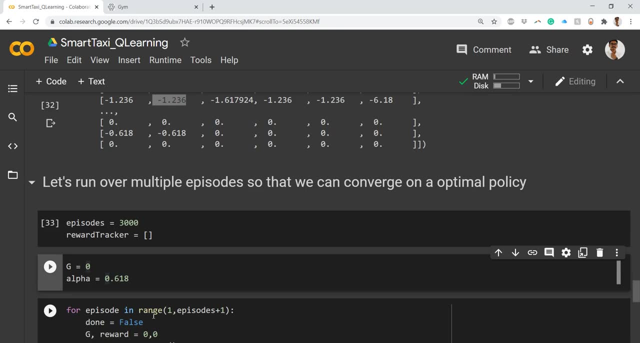 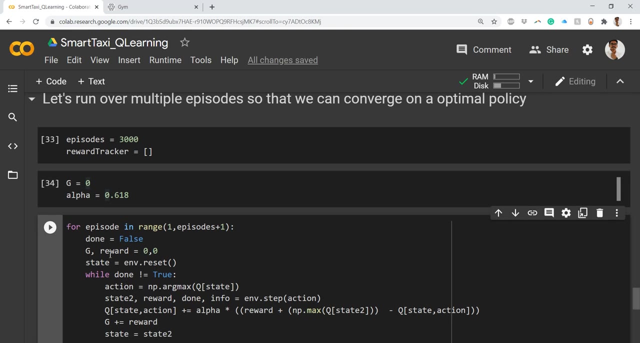 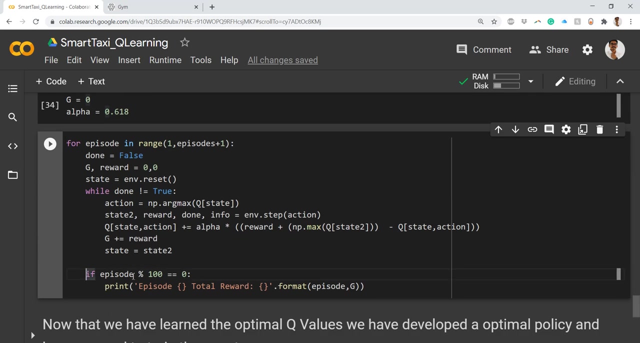 learned from all the 3000 episodes. so that is what the reward tracker signifies. the goal state is zero alpha. again, i'm taking it as 0.618 and then i'm just running over the same loop block again. so entire thing remains the same. and what here i'm doing is if my episode 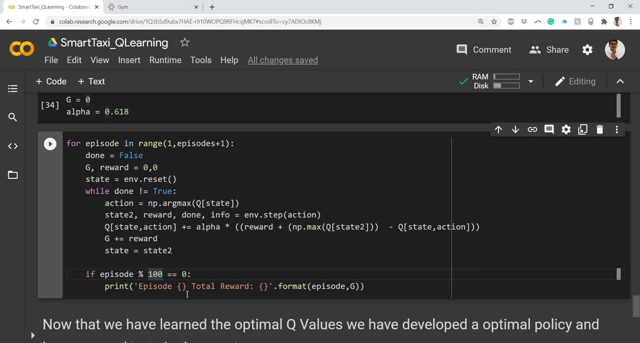 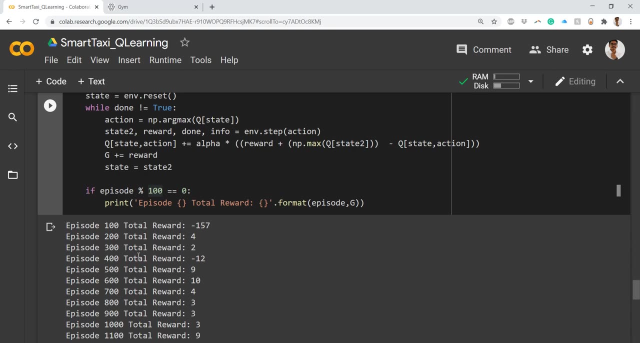 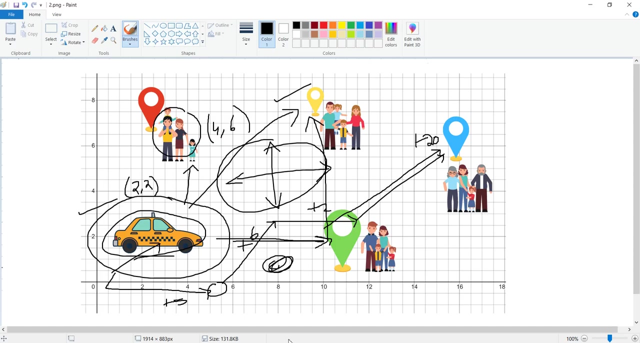 uh, mod 100 is equal to equal to zero. so i'm checking the remainder. so from every episode i want to get to know, like, uh, what is my reward? so that is nothing, but in one episode i'll get one reward right. so at one particular position, say when i went from this particular position to here. so 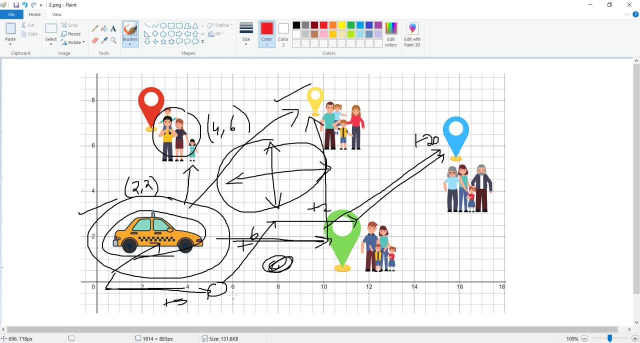 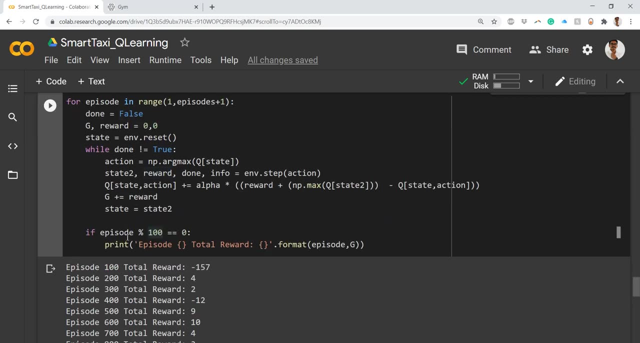 okay, in this particular scenario I get a plus 5 reward, in this I get a plus 6 reward, in this I get a plus 2 and in this I get plus 20. so I just want to print all these things. so episode mod 100 is. 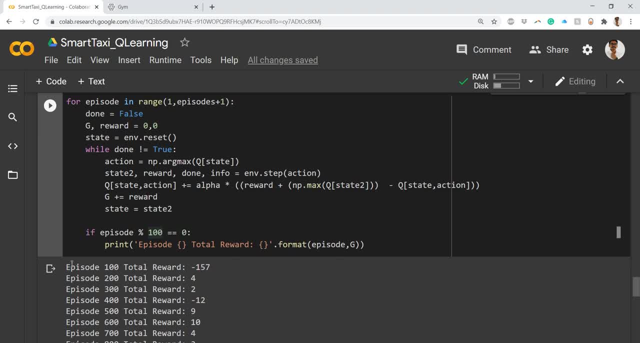 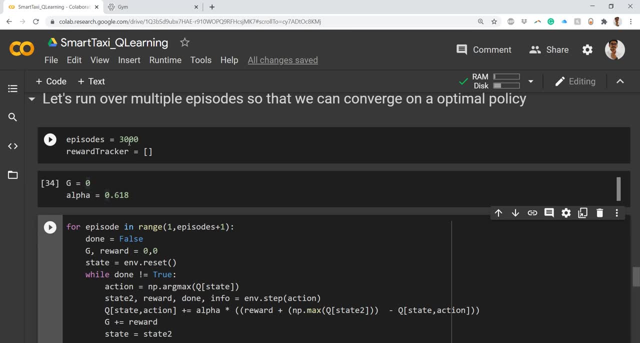 equal to equal to 0. so in the first episode, that is, on the 100th episode. now, since this is 3000, it is too much, so we are not printing episode 1, episode 2, episode 3. we are not doing that instead for every 100th episode, after every 100th episode. how much cumulative reward we are. 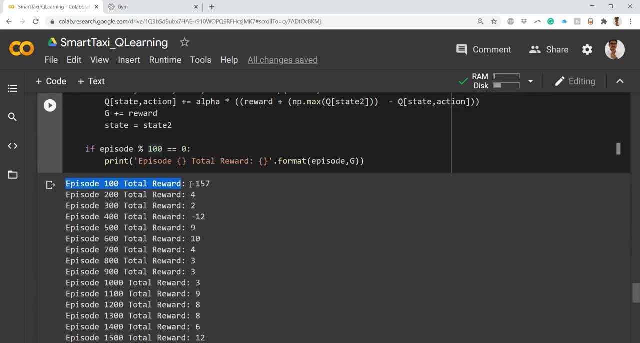 getting. so we want to get that. so it will basically print the list of that. so in the very first 100th episode it has accumulated a reward of minus 157. in 200 it has 4,, 3, it has two. okay, so you have some positive rewards, some negative rewards, and until it reaches, 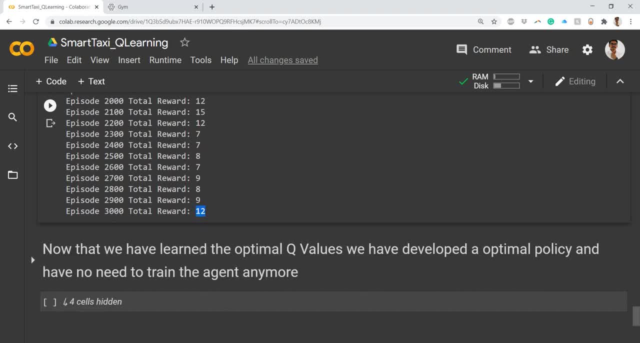 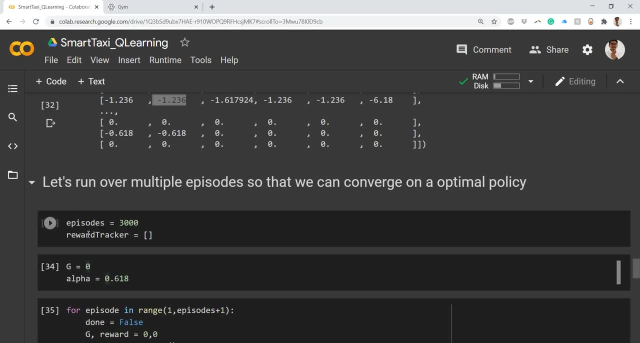 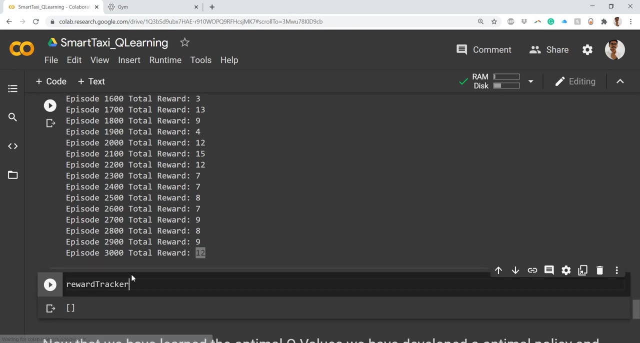 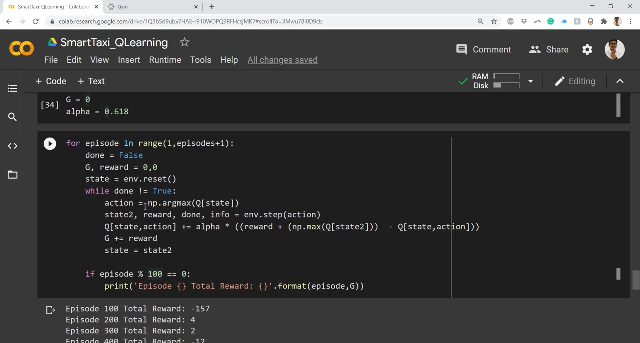 3000. it has a total of 12. so what we can do is we can just print this reward tracker and we can see whether, how many reward we have got so far. so it is empty because we are not appending this thing. we have just initialized this thing. we have to append to this reward tracker every now and then. 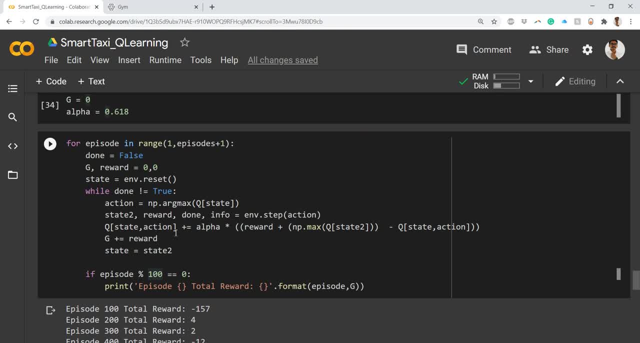 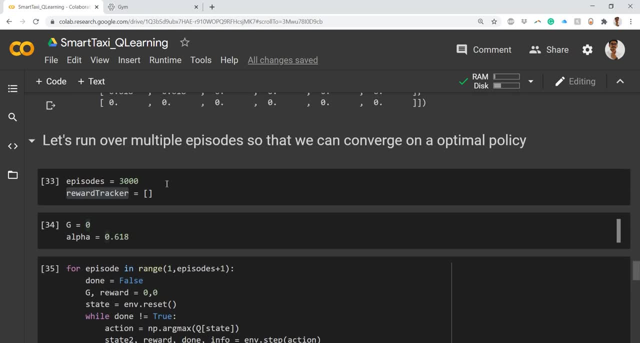 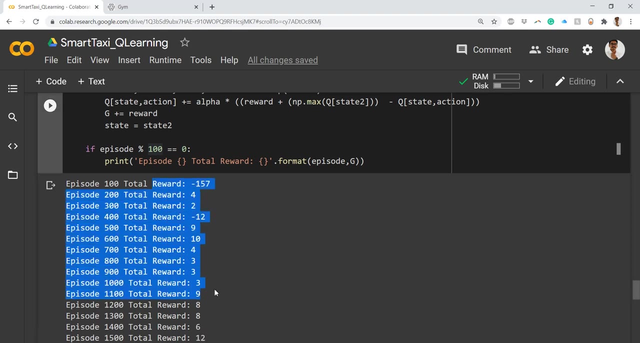 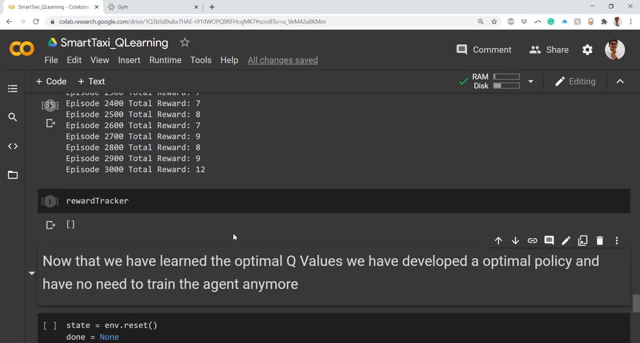 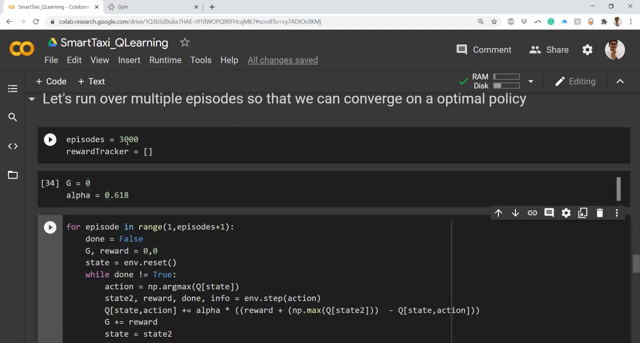 then we can get to know how many total rewards are there. this thing, since we are not currently updated, we have just kept a list of this, we have to append that so that same thing you can just make out from this particular steps. so, uh, so we can see it has maximized, so the maximum thing you can see, positive reward. so what if we did say: 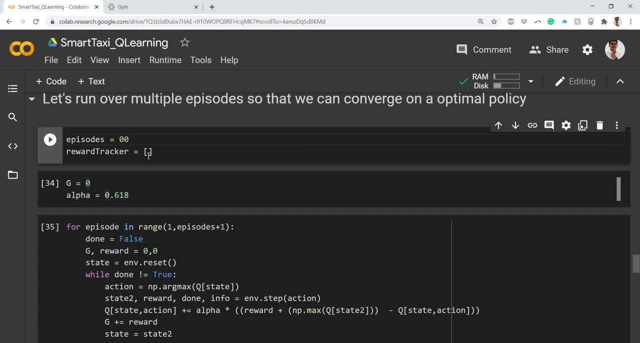 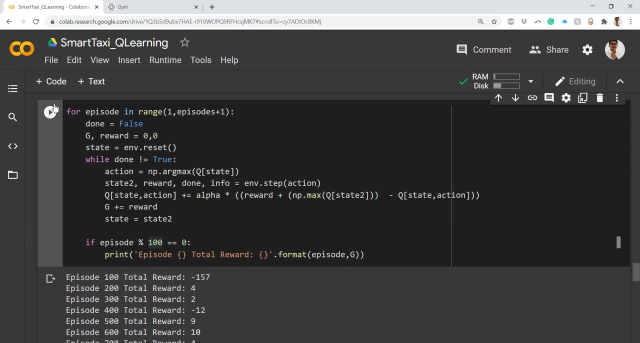 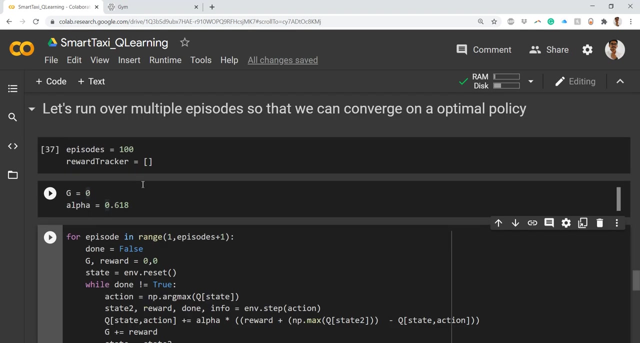 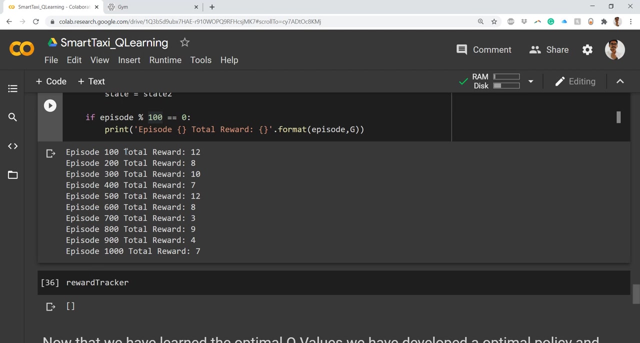 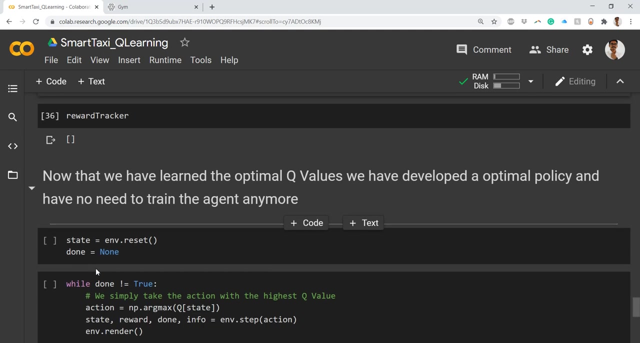 instead of 3000. we just only did some 100 episodes. so, in just 100 episode, because, uh, it is very small, uh, we'll keep it as 1000. we'll see how it changes this particular scenario. see, uh, we got all positive rewards and the best thing is that we want to visualize this thing. 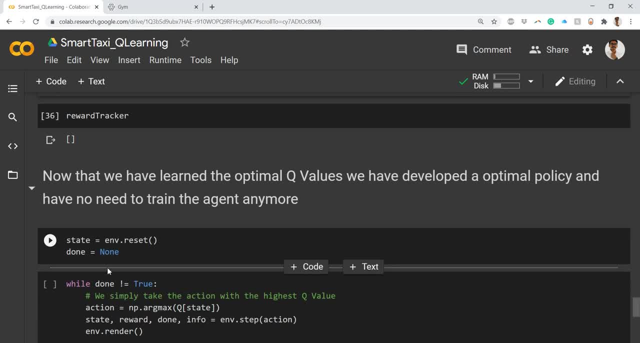 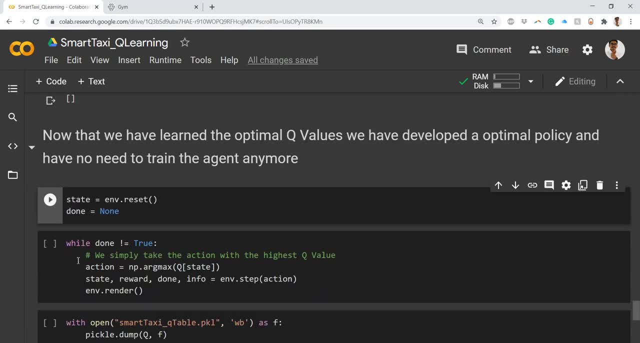 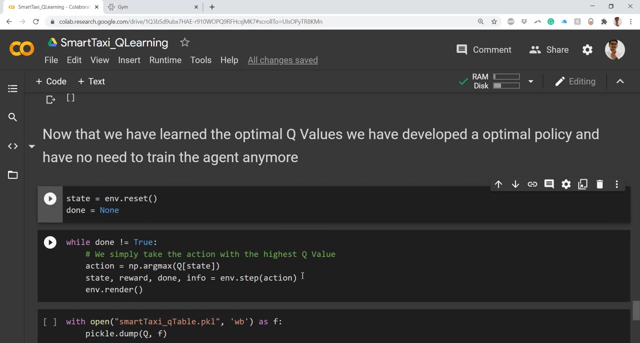 so in visualization we'll get to know at uh how the agent basically gets to know that the agent is performs this. so we just reset the environment. done is equal to none, while done not equal to true. so we take the action with the highest Q value. so if we 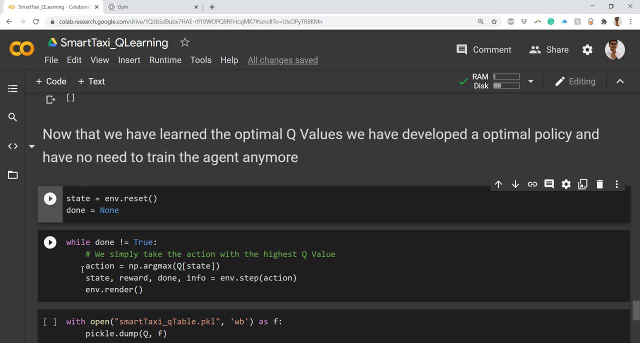 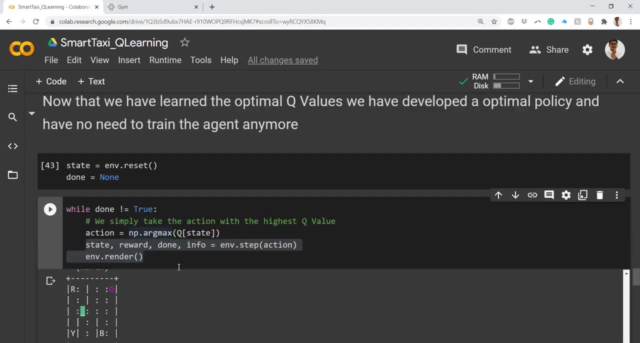 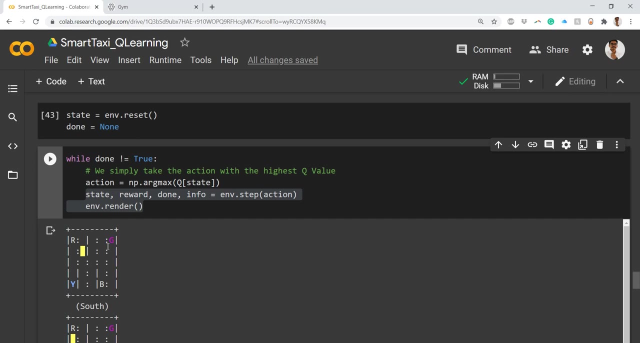 have the highest Q value. we go with that and we have this simple thing. so it follows from the above. so all the same things are there. we'll just call the render function. so in the render, basically this is the initial setup, how it looks like. so you have R, Y, B and G. so currently you can see the bracket it is. 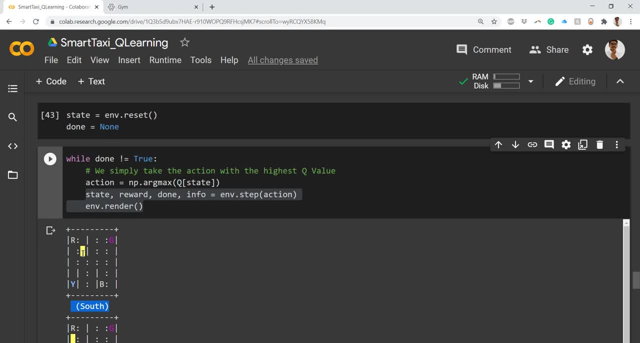 the location of that particular cap. so yellow represents your cab or taxi. so Y is the pickup location and G is the drop location. so first from this location you can see the drop location. so first from this location you can see particular position. it has to move to the left hand side. so for left we have 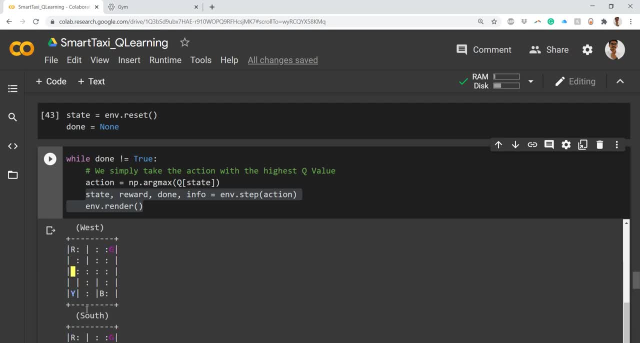 the convention West. so it will move to the West. it will again go to the south. okay, it goes to the south again. then once it is in the south it will do the pickup. so once it has picked up the passengers it has changed the color so now it is in green. so the cab you can see it is in green, now it is. 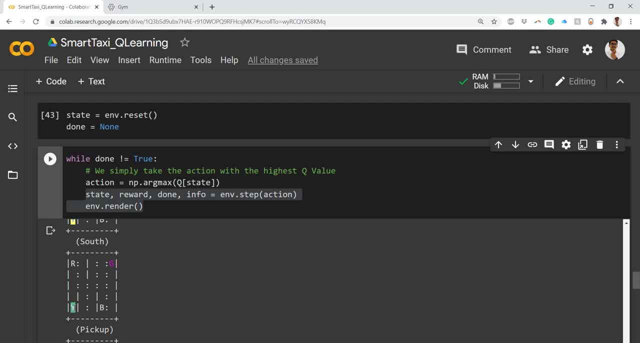 contained with the passengers. now inside the cab you have the passengers. so that means pickup now in pickup, with this green gap it is now moving up. so that is the north again to the east, so it can do the movements. so from this particular position it has moved north. now again it can move to north and then it can move to the 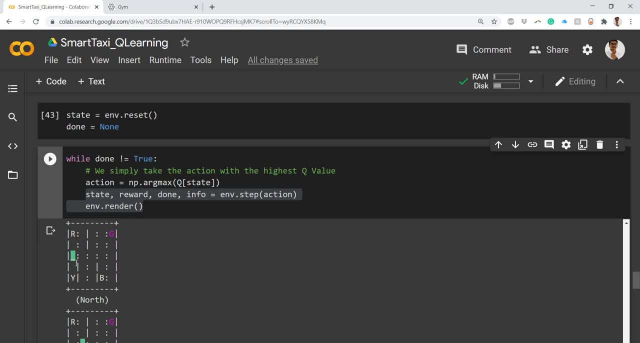 the east side and then it can go up. but it is done all internally, so it is making minimal number of steps and then it is trying to do this. so either if you move from one step again here or if you move to multiple steps here, so that has some kind of significant effects that will change. 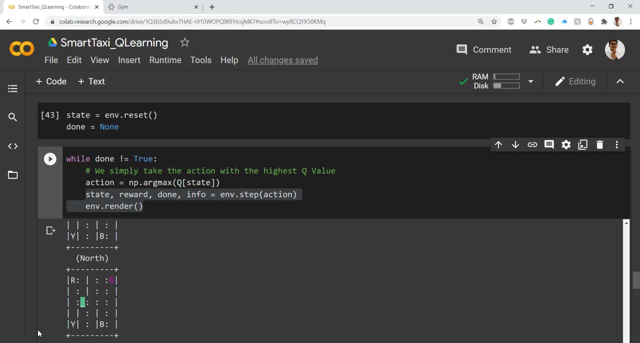 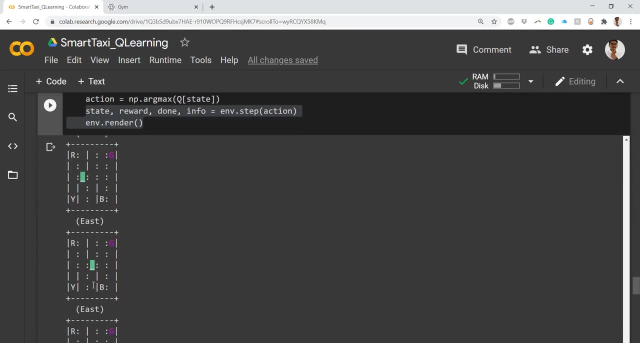 and see how it is affected with the help of the episodes. so it all depends upon the episodes. so now it is moving to the east, then again to the east, then, once it is reached here, now it has to move to the north. so it is moving north and north, again up. now it has reached the destination and 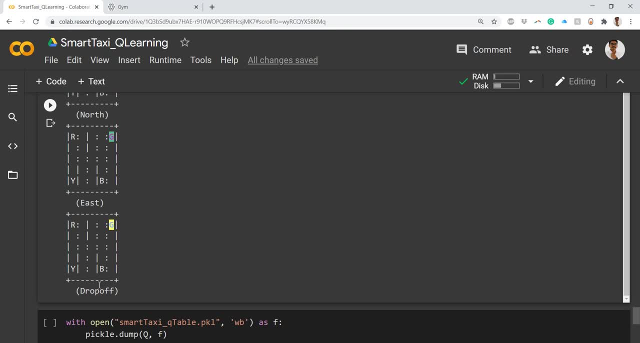 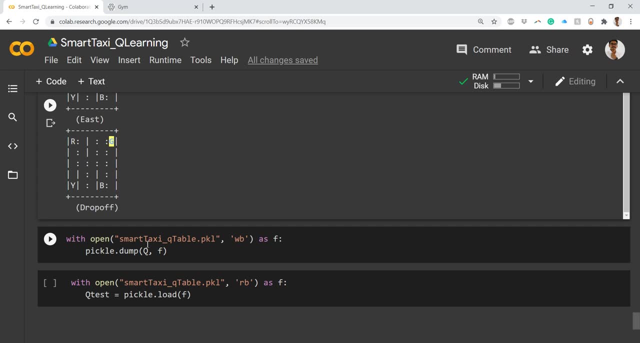 now the cab is again back to yellow state. so that is the drop off. so these two lines are nothing. but you are doing the object serialization that That is for object oriented thing. That is not much important. So you are using the pickle dot dump and pickle dot load. 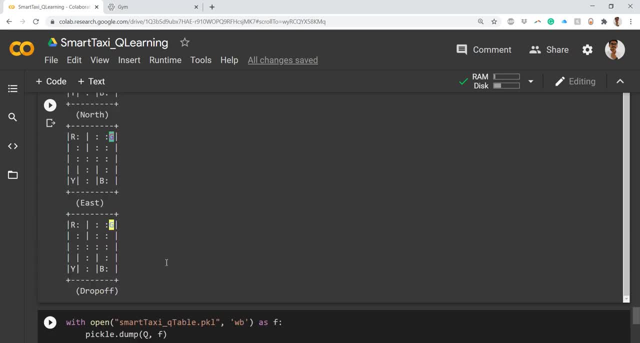 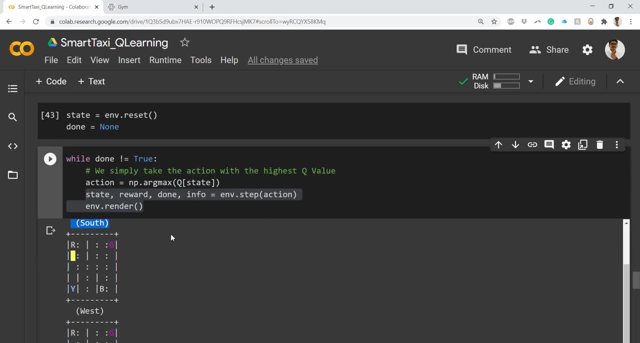 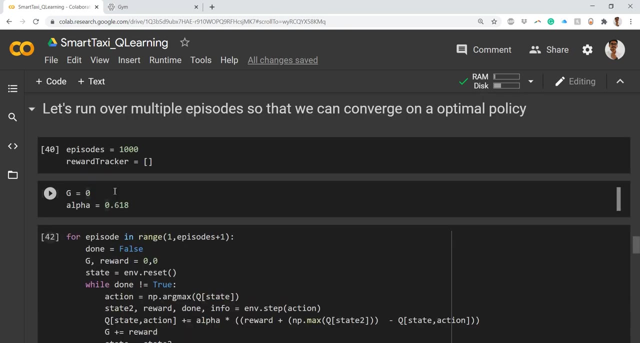 So write binary and read binary in that format. So the major thing that I want to bring to your attention is the convergence. At what particular point of time will this particular algorithm converge? So that heavily depends upon how much your episode is. So now, instead of say 1000,, I have 5000 episodes and we'll see how does this affect our Q learning. 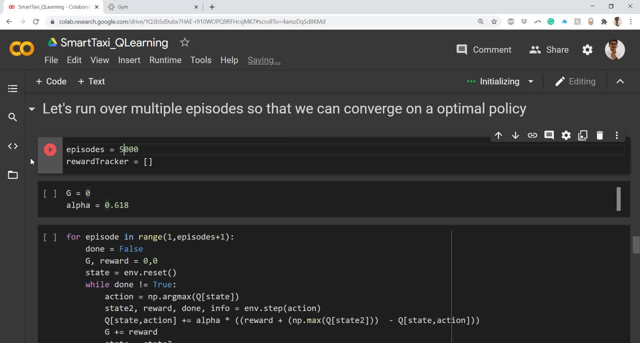 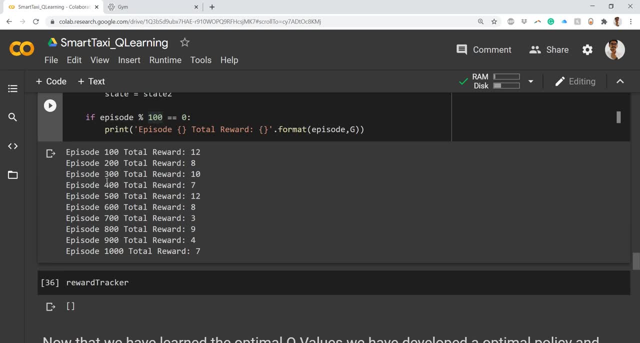 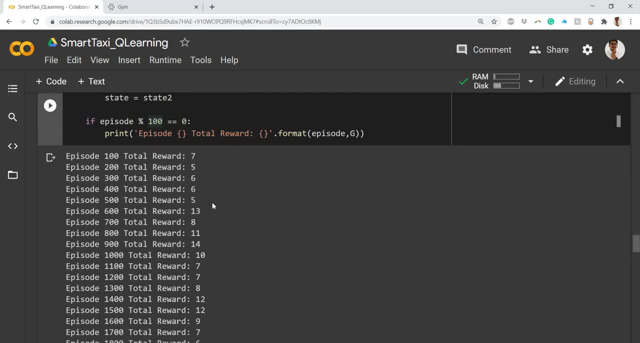 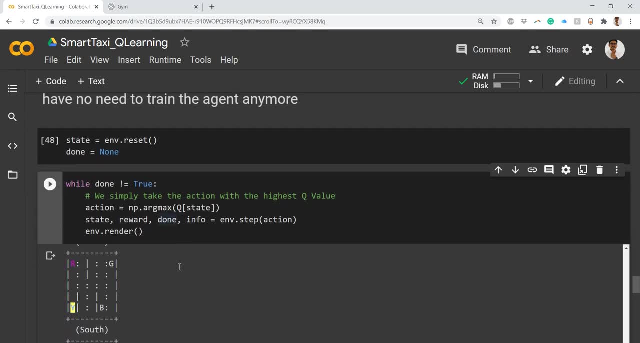 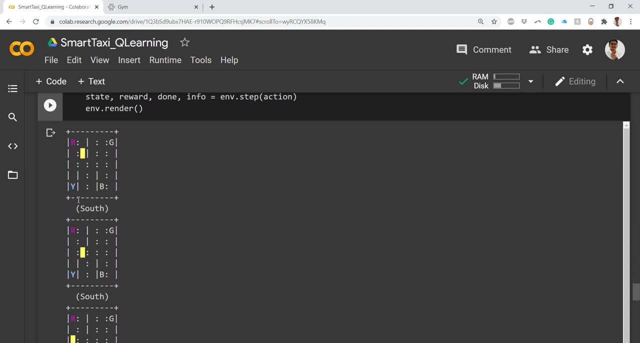 Okay, So we have all the maximum rewards and we'll just run this again. Okay, So now it is in the south, then south. So here also the pickup and drop location is completely upon the environment, So it is just random. So here the pickup is at the cab. 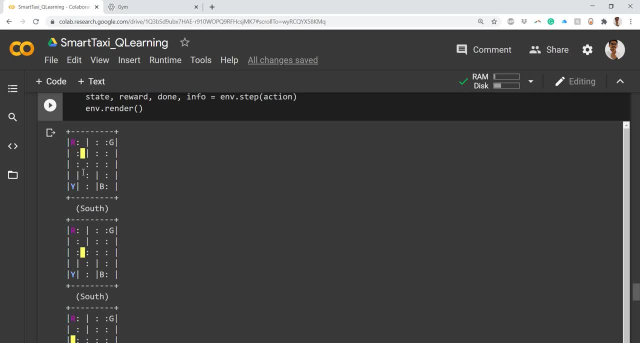 Generally was at the location at this particular point of time. at this coordinate It has to move to south in order to pick up the passenger. drop of location is at the red, So it will go to south, Then it will move to the west.